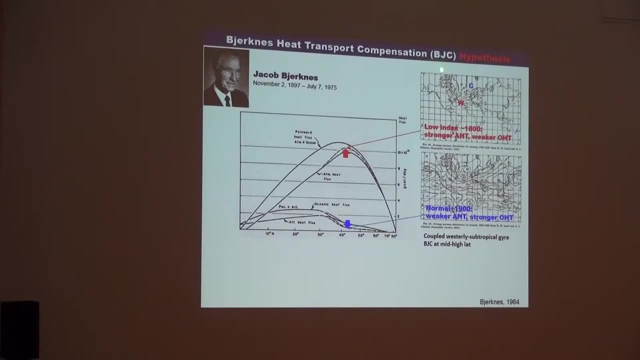 that in the early part the atmosphere. he can construct it from instrument data. It's called the low index. That is you have. it's not very straight, It's kind of a very meandered meridional direction, greatly And so and and the obviously in the 20th century it's. 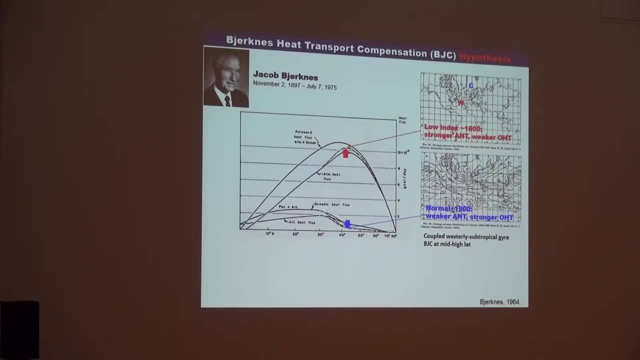 very straight, very strong jet. So then here's, here's his hypothesis. He thinks in this case it was because atmosphere transport more heat, because it go meridional more easily, Atmosphere transport more heat, But the ocean transport less heat because you have weaker 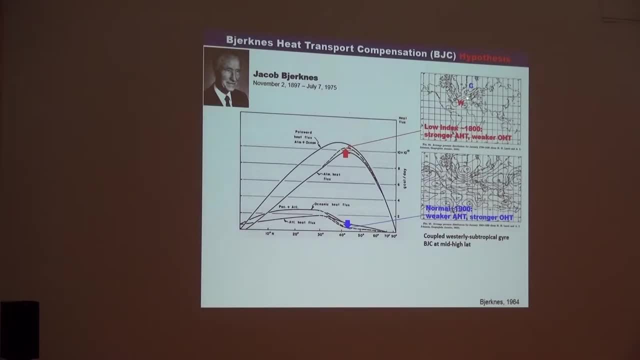 wind, So the Gulf Stream is weaker. So therefore you causes warm and cold pattern like this. Okay, So later it was opposite. Wind is stronger this way, So you have less atmosphere, heat transport, but stronger wind, increase Gulf Stream, increase heat transport, You warmed. 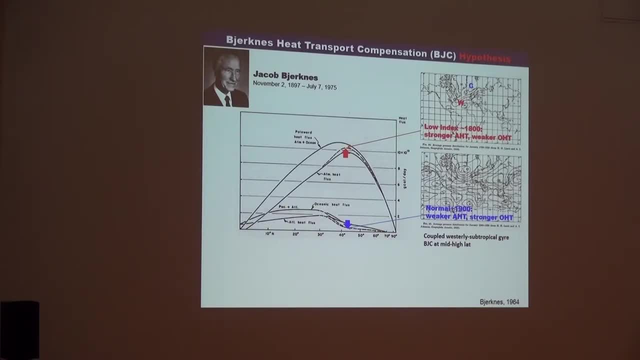 it up on the northern side. So he causes in this case you can see that atmosphere and ocean they go opposite. Now so he he put it here, He speculated the atmosphere maybe increase heat transport, you know, ocean and reduce heat transport. 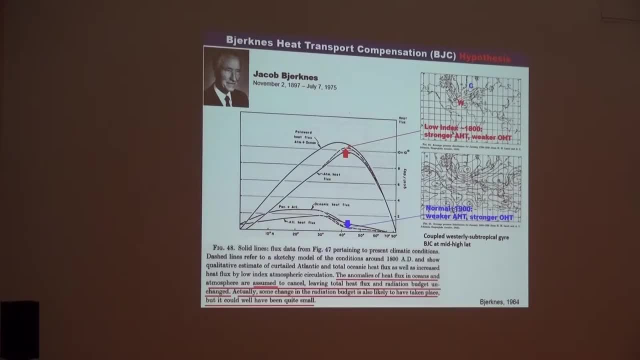 And vice versa, between these two scenarios. Okay, Now it should be emphasize that it is a hypothesis, because you look at his. his caption said that he: anomalies of heat flux in the, in the, in the ocean and atmosphere are assumed to cancel leaving. well, if total. 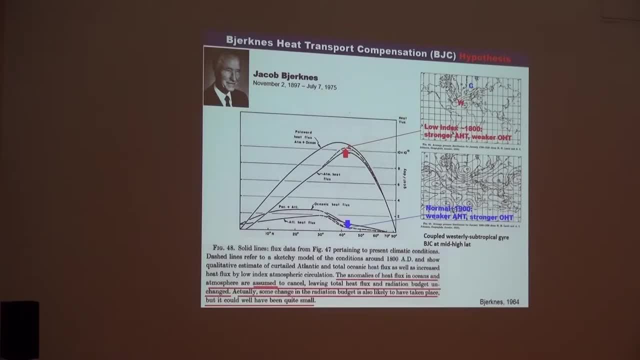 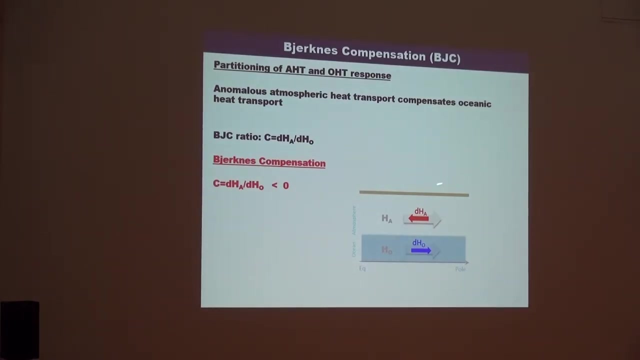 heat flux and radiation on the top of atmosphere, Your method of change. Okay, Thank you. Okay, so he doesn't know what happened, He just he thinks like this. Now think about this: If you have- let's suppose you have- no heat exchange, 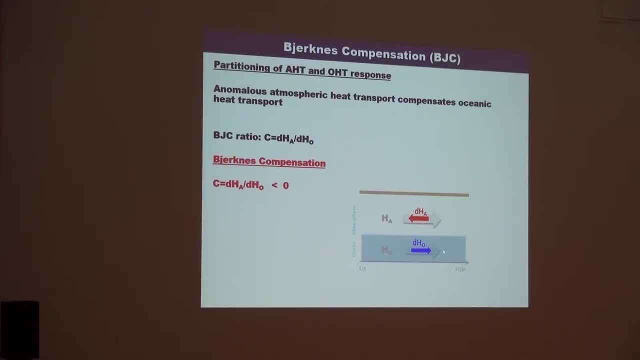 between top of atmosphere with the rest of world. Whatever happened here, of course you have to compensate, Right? that's very obvious. If I have no heat flux left here, if your ocean goes this way, atmosphere has to go this way, okay. 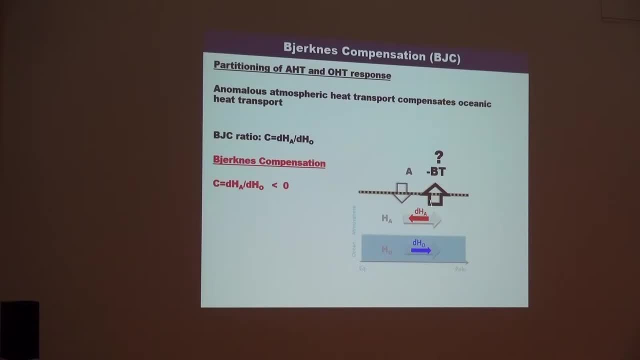 But now our real world. it's not like this. Because we have radiation from top of atmosphere radiates out, short wave come in. So our top is a leaky top. okay, It's not an energy flux zero, So therefore it's actually not obvious. 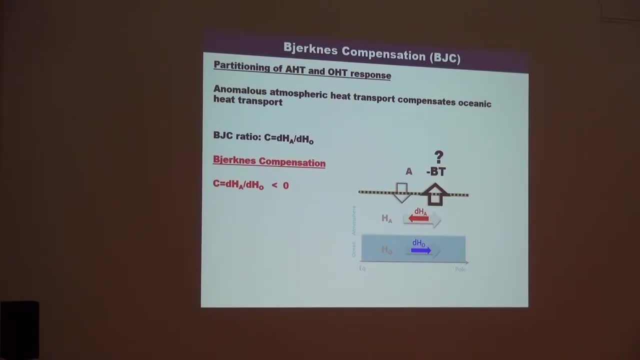 when you have the ocean go this way, does atmosphere have go this way? It's actually not very obvious, okay. So this we call the Bjergens compensation and the atmosphere, ocean heat transport response, that's delta, and if they go opposite direction, 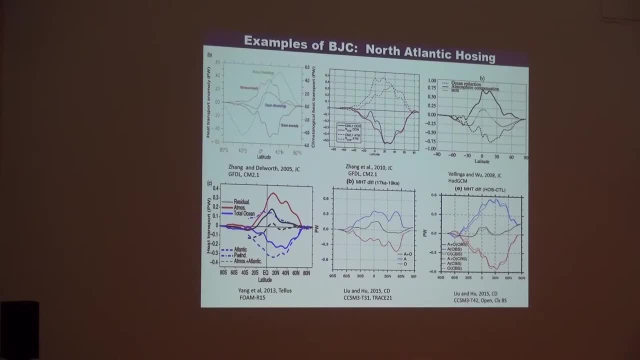 it means it's compensation. The question is, how does that happen? Now, in climate models we often observe that they are so robust. the same compensation. They just give you all the examples from different model: GFD model, In-car model, German model, whatever model. 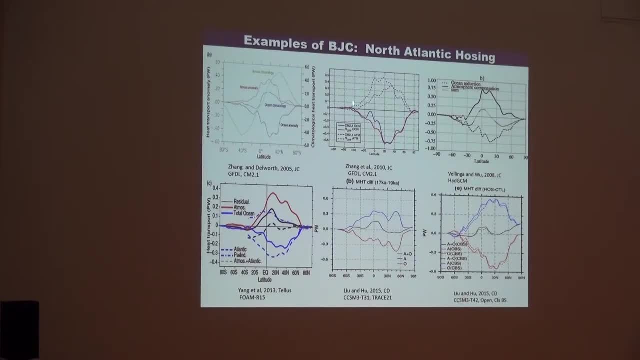 So why is this latitude? Why is atmosphere heat transport? Why is ocean heat transport? You see all of them. This is like in response to melting water in Greenland, AMOG collapse. You see all of them. When the ocean heat transport reduced, 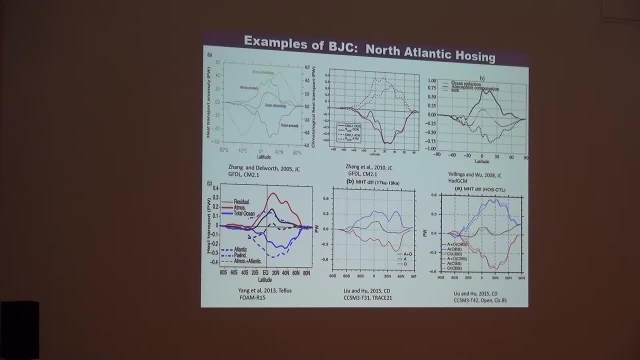 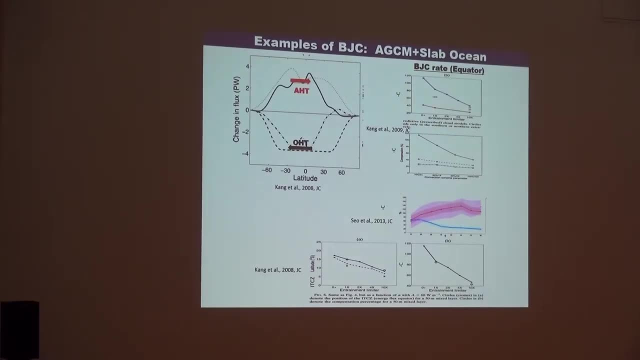 and when the heat transport increased they're always opposite direction okay, So in model they found that it is very robust. There's another type of model. I think Tony did this kind of model, a lot of this kind of model for this problem. 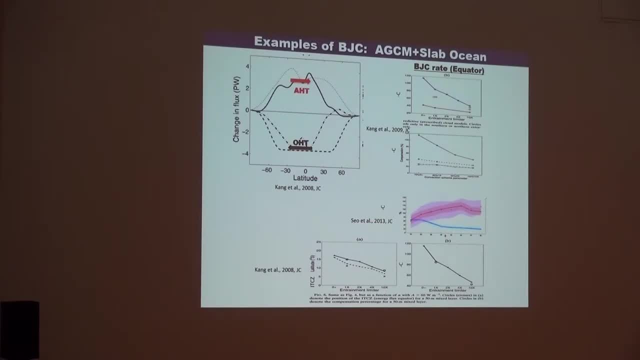 is that you use a slab ocean. That means I prescribe ocean heat transport, convergence through surface heat flux to the atmosphere. Then watch what is the atmosphere: heat transport respond Okay in this model. just give you example. right, If I prescribe heat this way, come out, convergence out. 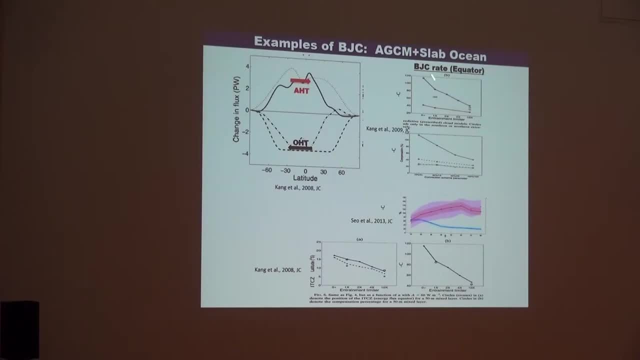 the atmosphere goes the opposite way. okay, This compensation, This, all of the examples showing different parameter regime, they all show compensation. okay, opposite. Now it's even more interesting to look at this. This larger than one means I have ocean heat transport this way. 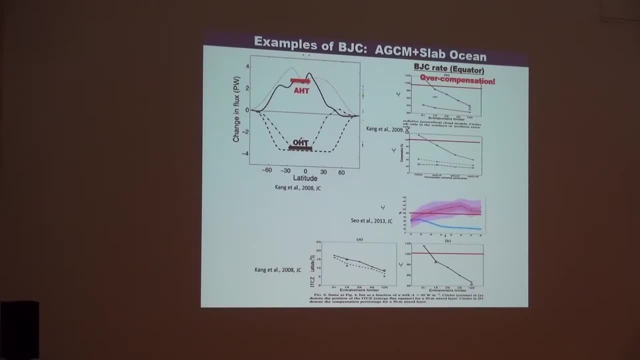 I have atmosphere heat transport even more than you have ocean heat transport. okay, So that's kind of okay. So that's kind of okay. Not obvious, right? How can I have more? okay, So the point is that the model 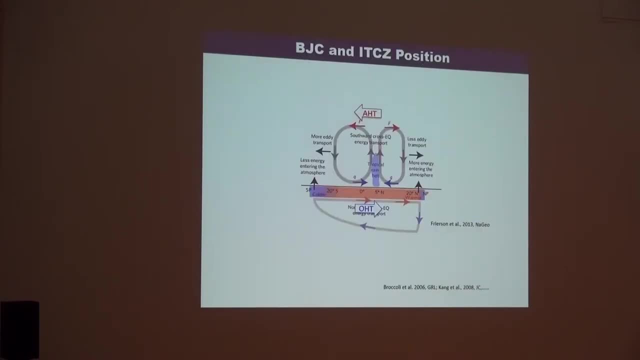 show lots of compensation examples And it's also related to a very interesting question people have been getting interested in. I think, Tony, probably one of first thought about this is that okay if you have ocean heat transport- let's say thermal heat line- changes transport. 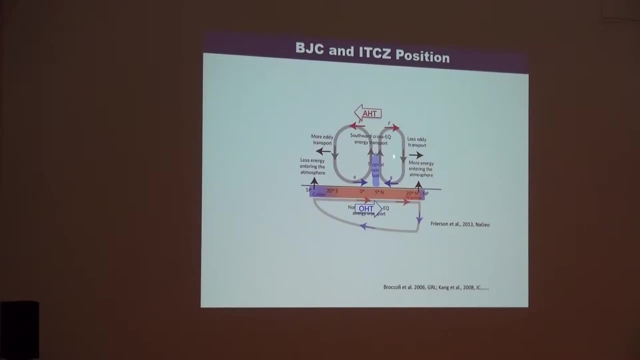 Let's say thermal heat line increase this way, Then assume atmosphere go the opposite direction, then the entire hardware system, the entire hardware circulation has to shift, okay. So therefore it's related to, for example, why the ITCZ, the intertropic convergence zone. is to the north of the equator nowadays. One argument is: because of the landing transport too much heat in this direction. The atmosphere has to go this direction. To do that you have to shift ITCZ to the north of equator, so the atmosphere, energy, is transported. 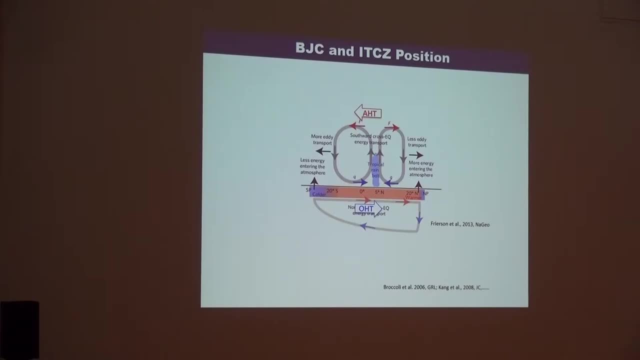 out of the upper branch to the south hemisphere compensate Okay. that's under the assumption they can't, okay, but under the assumption they compensate okay. Now we also have examples where they don't have compensate. Very simple example, in this case, in natural climate. 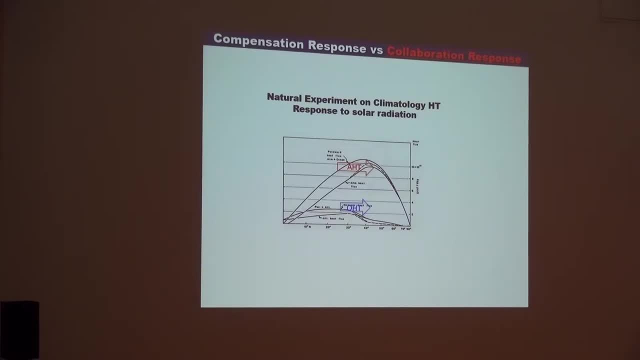 when I have solar insulation, come in. they both go the same direction. That's obvious. you know you have extra heat in the salt in the equatorial region. they have to transport that. At least that just says that you know. 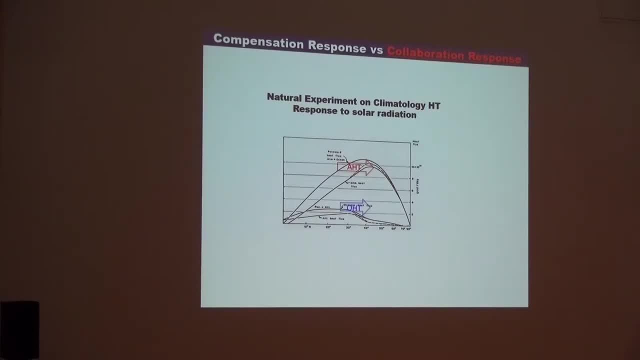 when you have general climate forcing, it's not always have to go the opposite direction, right, Even in this case. even in this case, I said there might be compensation, but there is a very robust mechanism saying that they may not compensate. there may be collaboration. 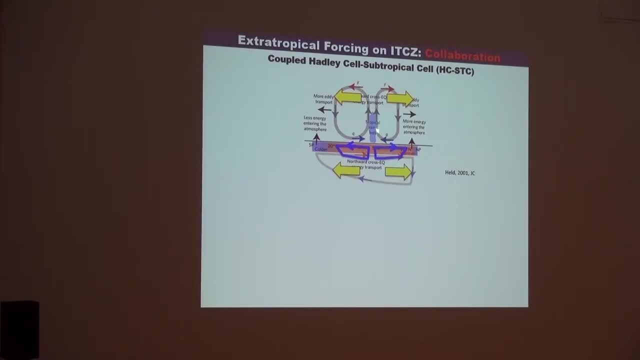 That is this coupled with hazardous circulation and subtropical sail. When the hazardous circulation's strong, the trade winds strong, you blow the ecmon wind stronger, then you blow the stronger subtropical sail. so now the hazardous circulation: transport heat to the north and forward. 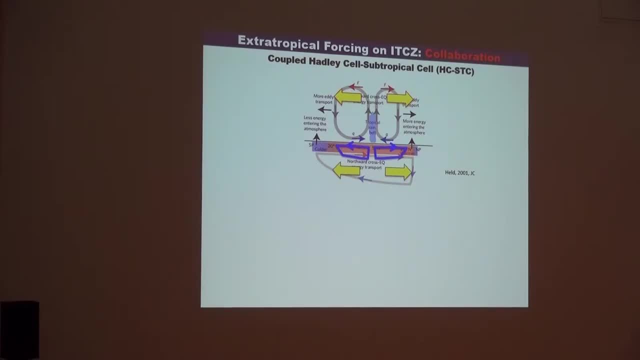 the ocean also transport heat forward. so this action actually is a collaboration mechanism, very robust physical mechanism. So the point is that they don't have to always compensate. And recently there are more experiments, numerical experiments. they were trying to test when we have a highlighted climate forcing. 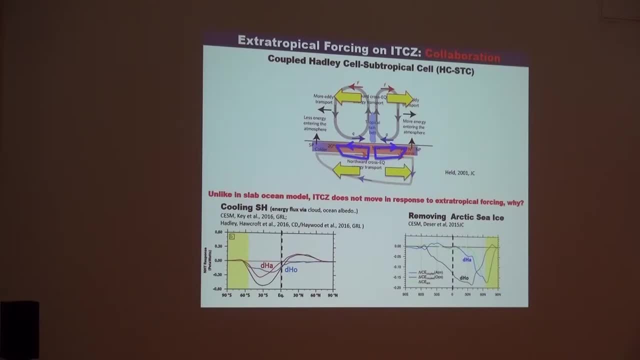 how does that affect tropical ITCZ? You expect they have compensation. ITCZ move a lot, but what you find in this fully coupled model is that there's very little response- very different from mixed layer model we talk about. See this example when you change the clouds. 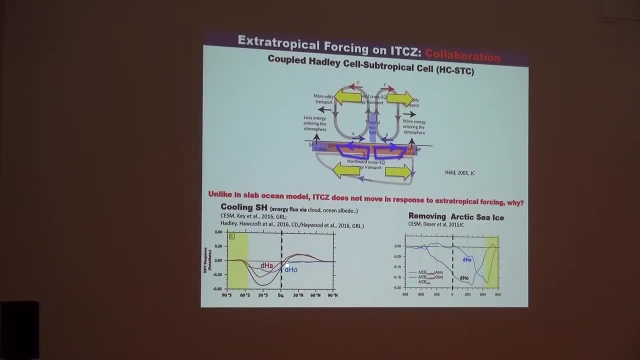 in the south hemisphere. look at the ocean, atmosphere, heat, transport. they are in the same direction and become very little. when you go to equator, They are not opposite. This is another experiment you did with NCAR model in Arctic: you change the sea ice. 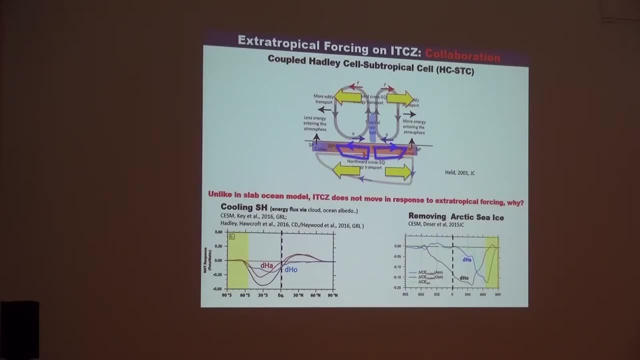 Then you see the ocean atmosphere heat transport. again, they are in the same direction and there's very little atmosphere heat transport on the equator. therefore there's very little change over the ITCZ. okay, So the point, the question that was raised, is that: 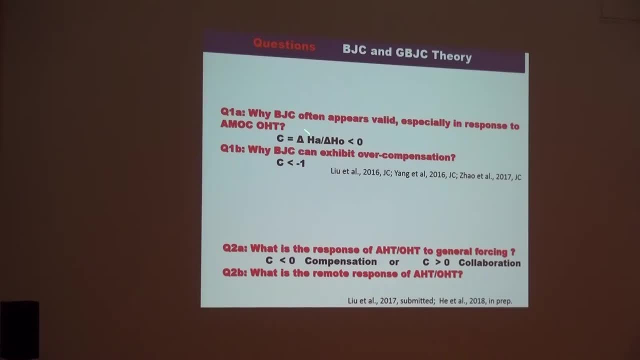 first of all, why in certain type experiments we have seen there, Biotic Discompensation is so robust. I showed you the first two pages, lots of examples- And but in the meantime why It seems like there are also other cases. 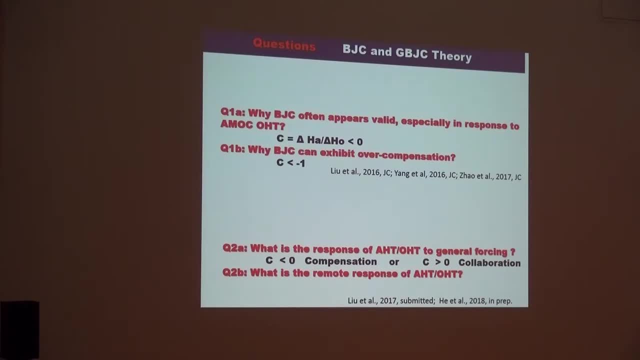 where the atmosphere ocean, they may not go opposite. So what is the condition? when you will have them? compensation, when you have them, collaboration right. It's a general problem, climate dynamics problem. okay, And in the first part of the problem, 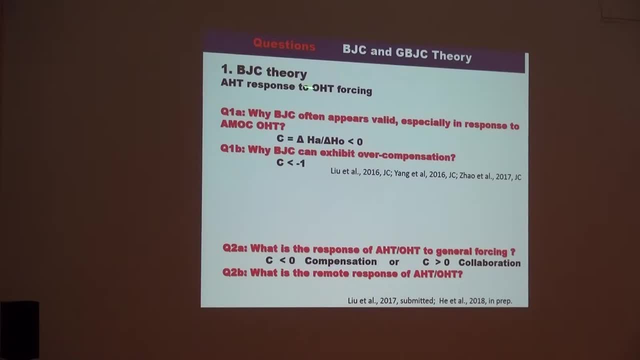 I called it the Narrow Sense Biotic Discompensation Theory. You want to know why it's robust. Also, you want to know any theory if you have have to know why, under some conditions, the atmosphere can compensate even more. 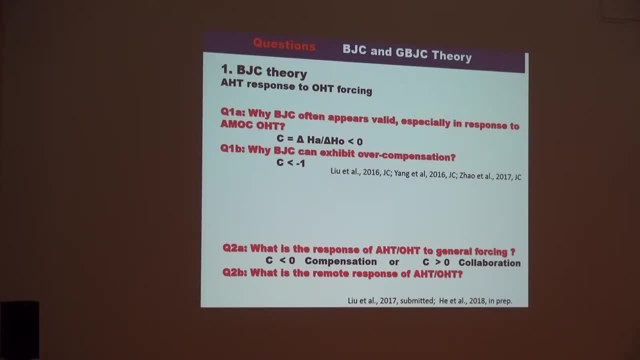 than you transport in the ocean. okay, Because we saw example And in the generalized Biotic Discompensation Theory. here we not only want to know what kind of forcing you produce heat compensation, We also have. another issue is that if I perturb at high latitude, 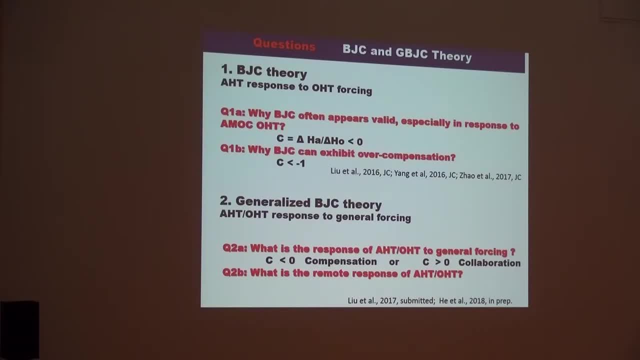 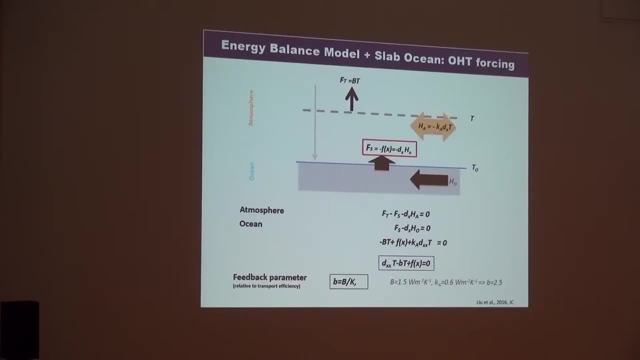 how does ocean animal heat transport in the remote places? Okay, so that's called remote problem. So let's start with the first one. In this case, we can simplify to start with slab ocean, because we're going to prescribe ocean heat transport. 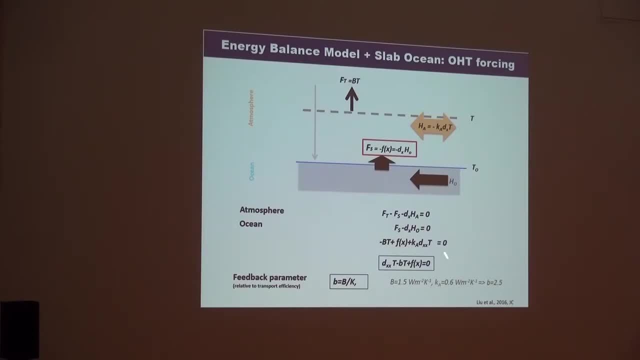 Watch: how much is the atmosphere response? okay, So we can use the energy balance model. That is very simple. You have the prescribed ocean heat transport in the ocean such that there's a convergence forcing the atmosphere, That's energy from the surface. 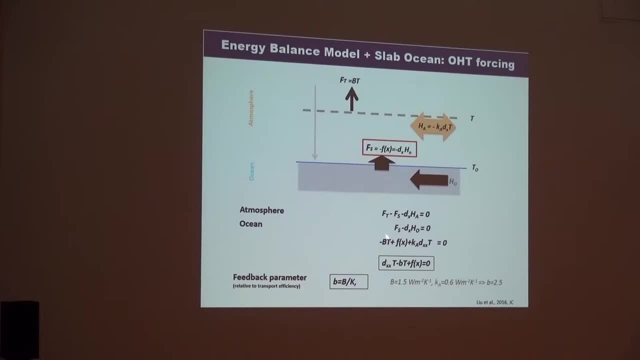 That this is from the surface, That on the top of the atmosphere there's a long wave radiation radiates out. That's a Bt radiates out. You get a warming, then it radiates out. Then the final thing is that 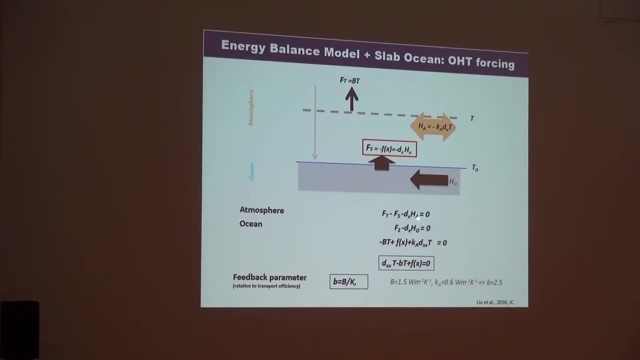 the rest will be the atmosphere. They have to be transported by the atmosphere. Okay, that's all energy balance model. okay, And in this energy balance you write it down Mathematically. it's basically order differential equation. second order differential equation. 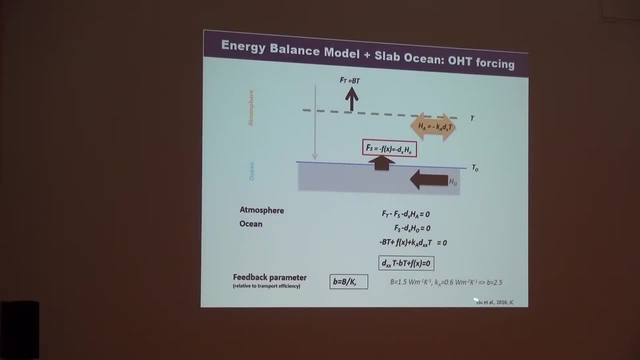 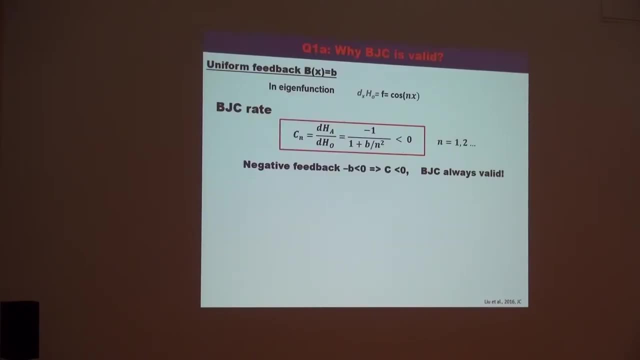 And the parameters. you can this B, especially the feedback parameter. you can ask the value about two or three roughly In this model. actually one is a constant coefficient. You can solve them analytically Because you use the eigen function sine cosine. 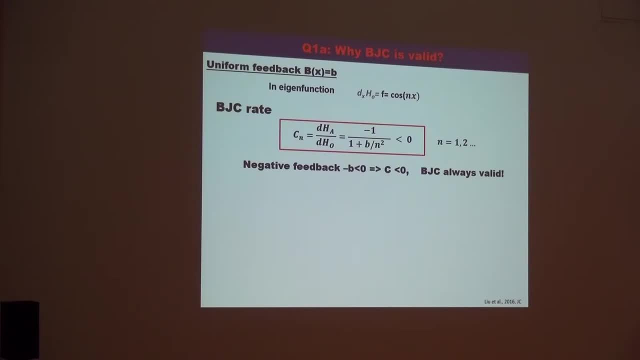 Or, in this first case, you use the Lagrangian polynomial. You can solve that, So you can explicitly calculate the reactance compensation ratio. That is, if I have ocean heat transport perturbation, what is the response of the atmosphere heat transport? 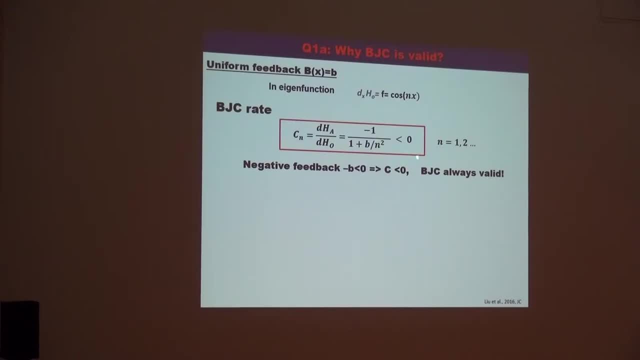 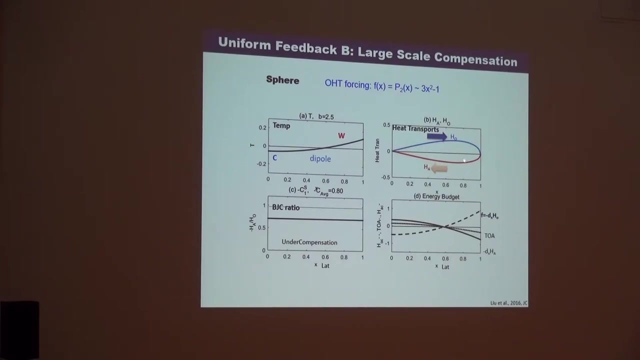 Then you write it down. That is the formula. First thing: always smaller than zero. okay, So in this model, if you perturb ocean atmosphere, always go the opposite. In this example I prescribe the ocean heat, this direction, this heat transport. 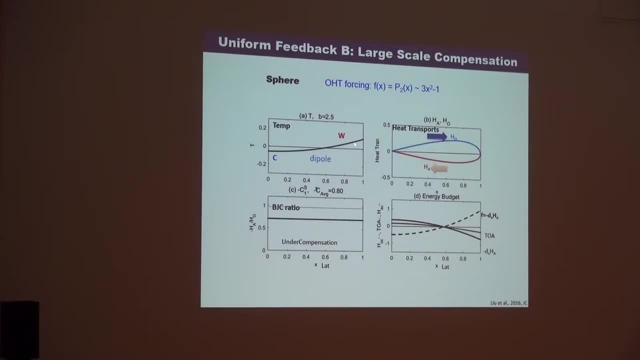 And then solve the problem. You find that it just warm up here very reasonable. You transport the heat, warm, cold And ocean, sorry, atmosphere transport, opposite direction, Okay. And you look at the heat budget and it's balanced out by the, the ocean heat, okay. 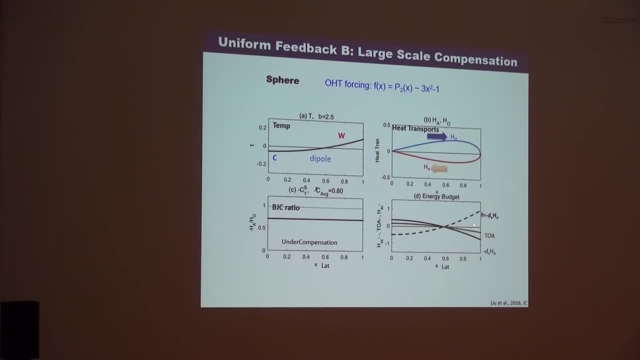 The ocean heat transport is balanced partly by the top atmosphere radiation, partly by the ocean atmosphere heat transport, And the ratio is about. just we calculate in that formula. The mechanism actually is very simple. okay, Think about it. 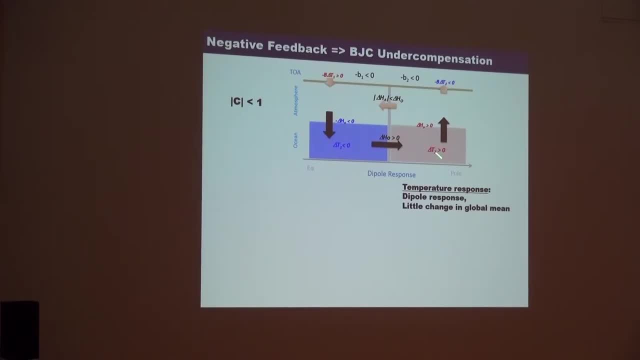 Suppose, in the coupled system I transport heat toward this region. okay, Well, ocean, all the ocean. heat has to come out. No damping in the ocean itself has to come out. Now you have two choice. Part of it is damped because you have the speed. 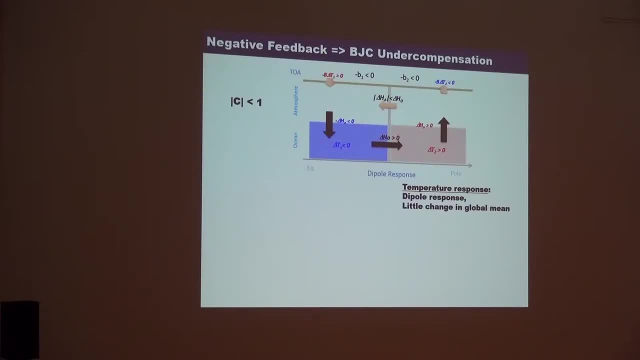 larger than zero means there's a negative damping to long wave, damping to the top of atmosphere. So you damped out. Well, you damped out, then the rest will be transport in this direction. So you have to go opposite direction. 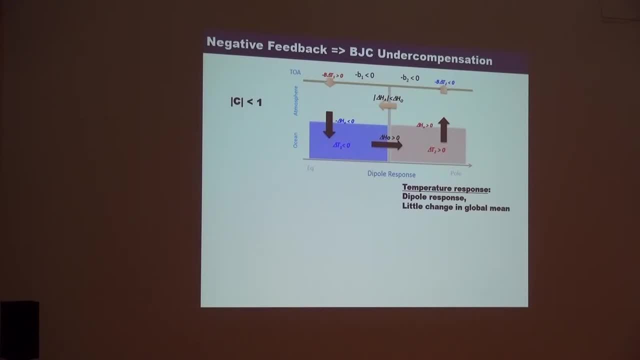 from where you prescribed ocean heat transport. So they have to be negative And you can see the spin-up process. When you suddenly start heat transport in the ocean, the atmosphere goes the opposite direction, And so the temperature. so the north part. 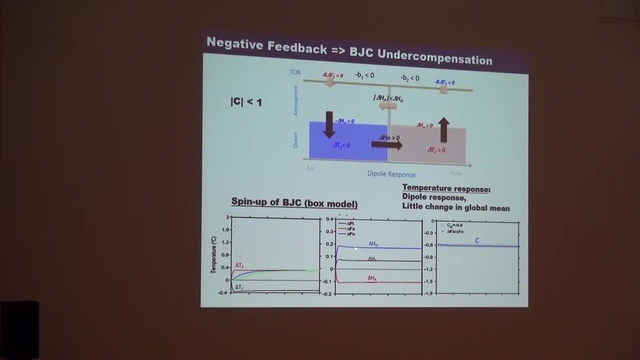 warmer source cooling and the heat transport atmosphere just opposite to this, okay, And the reactance compensation ratio with time is always negative in this case. So the mechanism is actually very robust. Now let's look at it more quickly. 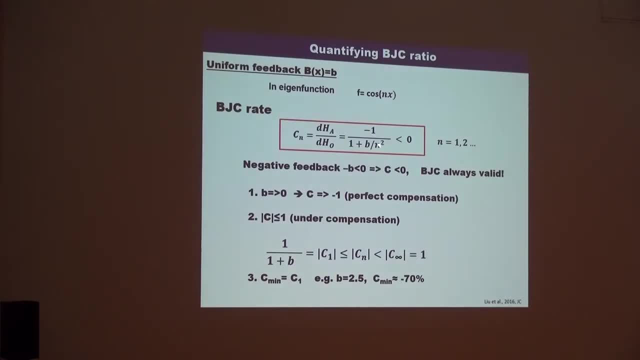 More carefully. quantitatively. Look at this formula. okay, Now, if B equals zero, C equals minus one, What is? B equals zero? B equals zero means my atmosphere does not radiate heat out. That's like rigidly. 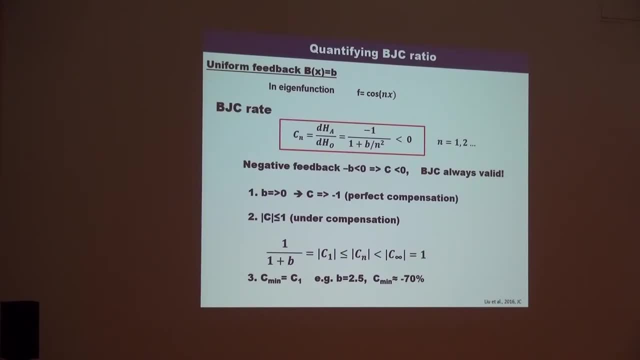 That's obvious. Whatever heat come in the ocean, exact amount has to go out. That's why it's a perfect compensation. It's one okay. Now it is interesting. Well, in real world we have damping, long wave damping. 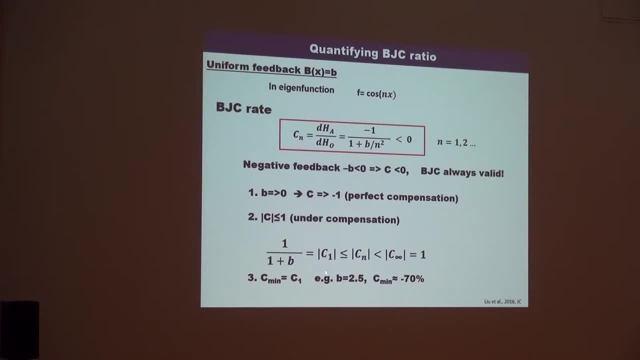 So it's not a zero, So it's positive here. Now, in this case the minimum compensation occurred in N equals zero, N equal N, equal, yeah, N equal one, sorry, N equal one. That's a very large scale into atmosphere, heat, transport. 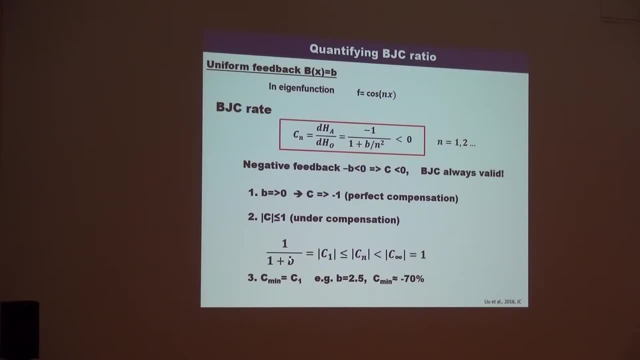 So that's minimum damping. Minimum damping it complete just depend on how big is it. It depend on ratio of the feedback. The feedback is about two to three, So you plug it in, it's about 70% compensation. 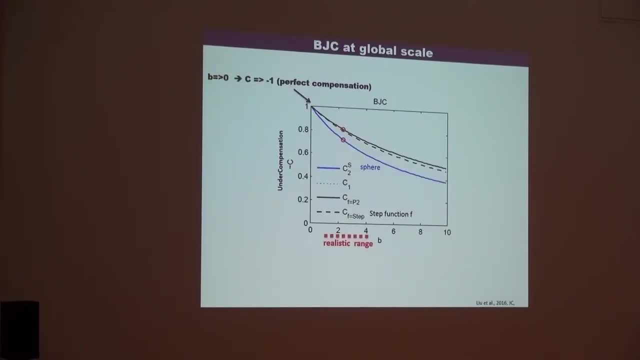 The atmosphere compensated about 70%. This, just one example, shows that the minimum compensation ratio as a function of this feedback parameter realistic regime is about seven percent, 70%. Now it's also interesting to look at this for small scale. For small scale, N is very large. 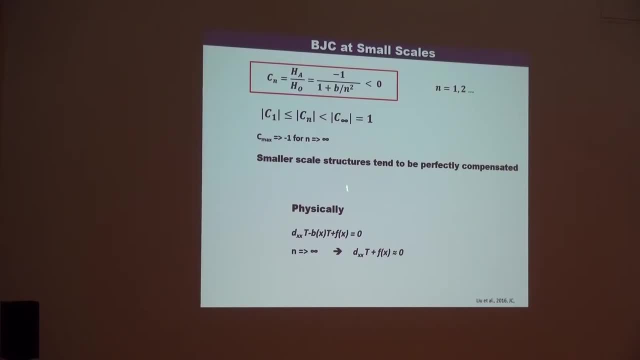 So this equals zero. This becomes a perfect compensation. It means, if I prescribe ocean heat, transport has very complicated structure. okay, I have heat coming up in a structure For this, the atmosphere, complete compensated, One to one compensation okay. 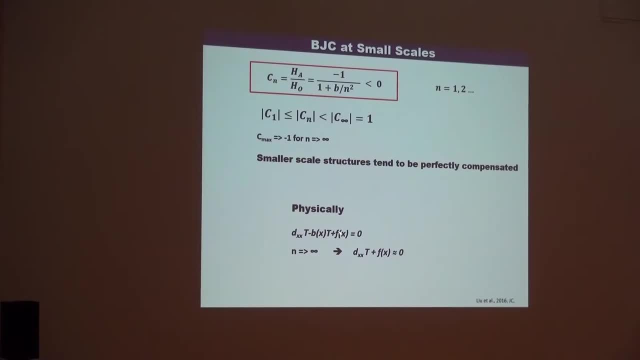 Now, mechanism is very simple. Think about this formula. This is the heat transport you prescribe as forcing. If the scale is very small, the derivative became very, very large. So the balance is between this heat transport conversion and the forcing. 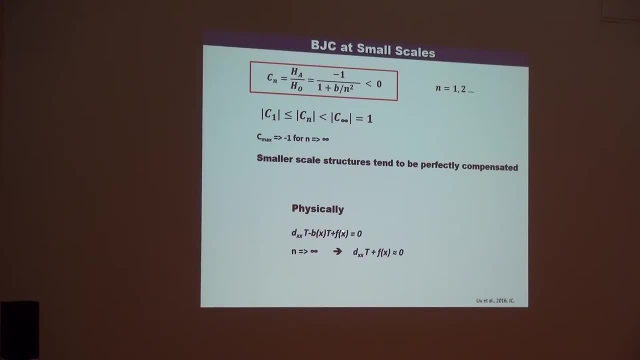 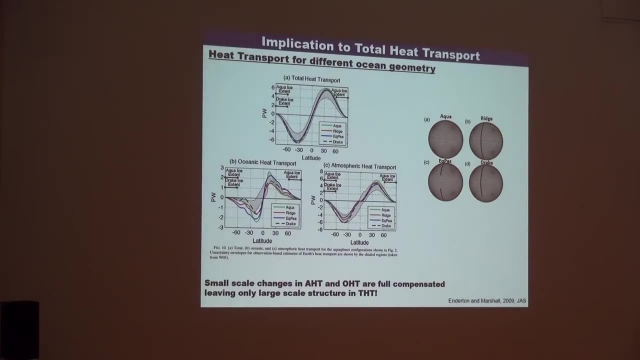 So the complete balance. So the forcing, ocean forcing is complete balance by the atmosphere, heat transport. That's why complete compensation. Now there are interesting examples, okay, And for example, in this case it was Marshall had some experiments. 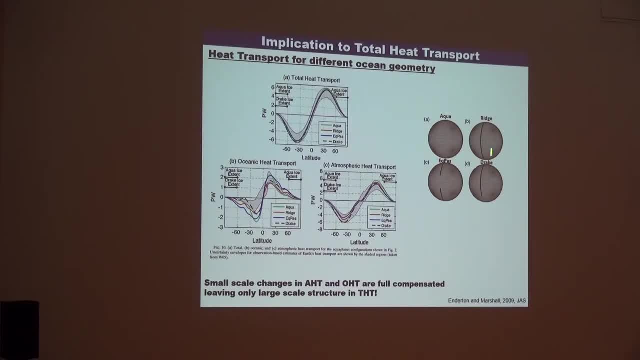 They used a coupled model, but it's idealized geometry, constant. My point is that you look at the global heat transport, total heat transport, very smooth, But look at the atmosphere and the ocean alone: Very wicky, okay, So they have very small scale structure. 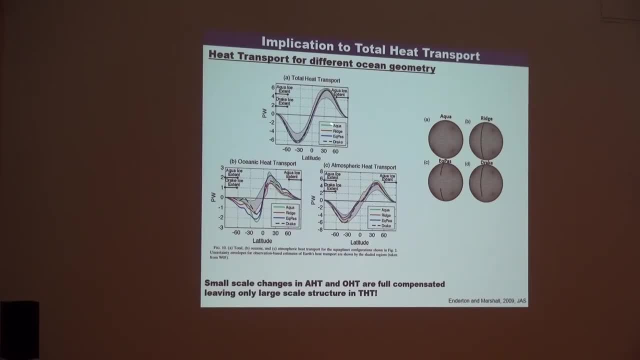 But the small scale structure when you add them together it's gone Because they are completely compensated okay. So that's just consistent with the theory we talked about before. So in global total coupled heat transport it's very smooth structure. 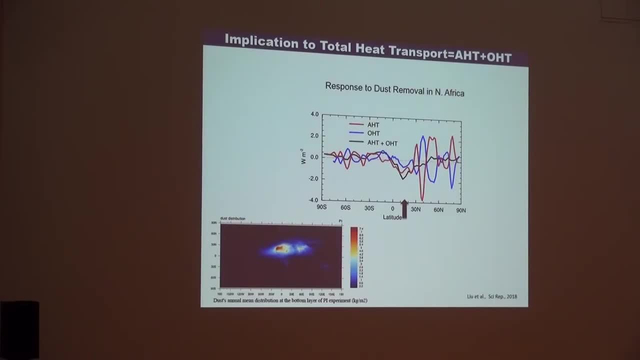 You don't have very little structure. Now this is another example we're doing. It's from some dust effect, of Africa dust, So we're putting dust here. see what happened. But forget about the other point I'm just looking at here. 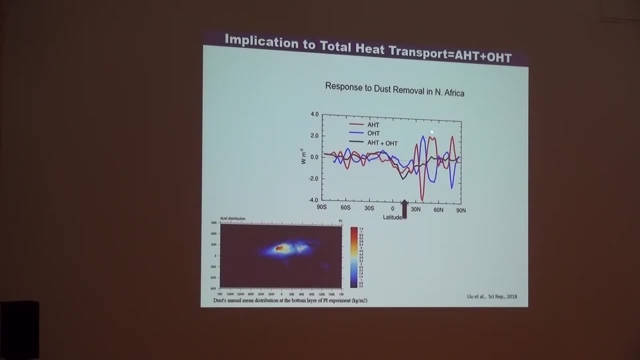 This heat transport anomaly produced by the dust change in Africa. The red is atmosphere heat transport anomaly, Blue is ocean. You can see that they almost a small scale. they just almost completely compensate. As a result, the black is a total. 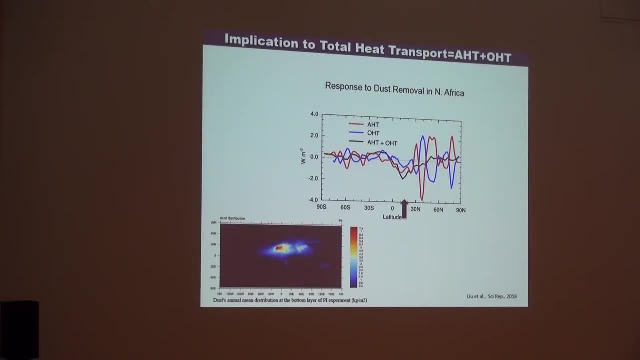 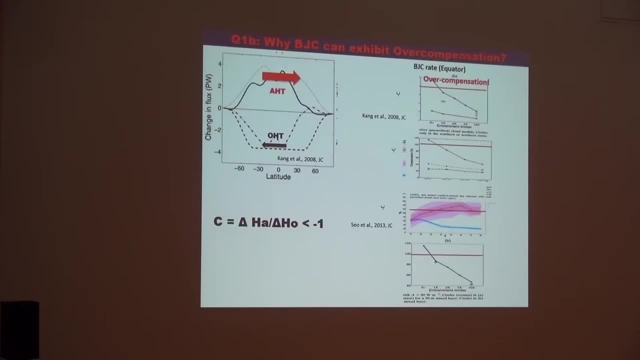 has a very smooth structure. okay, So high wave number, they tend to compensate. Therefore, in the total coupled global context they tend to be very smooth large scale. But we still have a problem. As I said, you have some parameter regime. 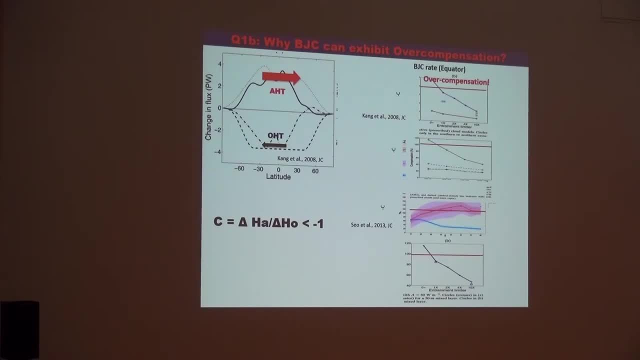 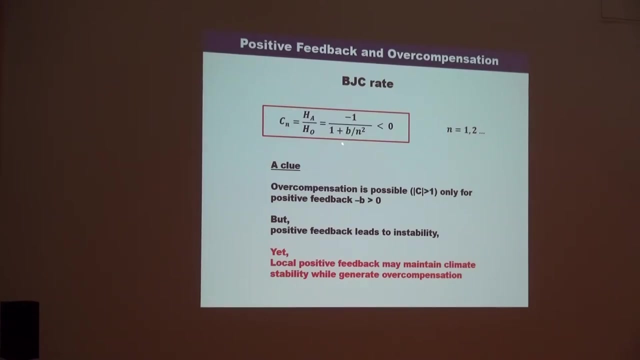 you can produce, even post, even over compensation. That is, you give ocean one watts per square meter, I can have two watts per square meter going the other direction. How can this be possible? Now start with looking at this formula. This formula: if B is larger than zero, 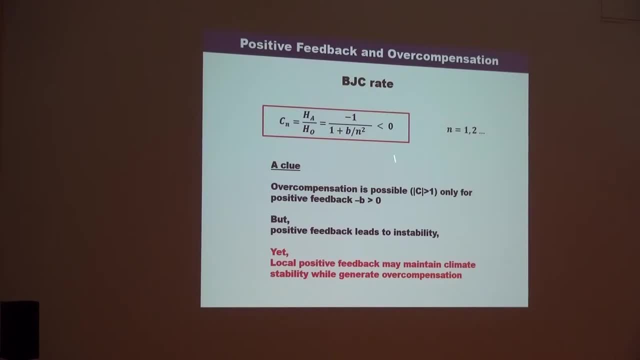 that means I almost damped atmosphere. This has to be smaller than zero. smaller Has to be smaller than zero, Smaller than one the value. okay, So you have to have the so-called under compensation, The only way you have over compensation. 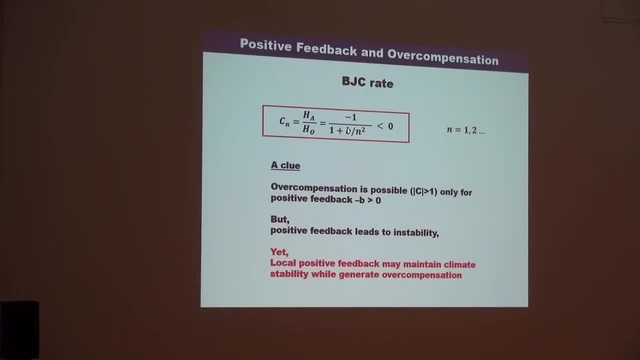 this value is larger than one, this has to be negative. B has to be negative. okay. B is negative means my top atmosphere is positive feedback, not negative feedback. Now you have a problem. Global climate cannot be positive feedback, Otherwise we have runaway greenhouse, okay. 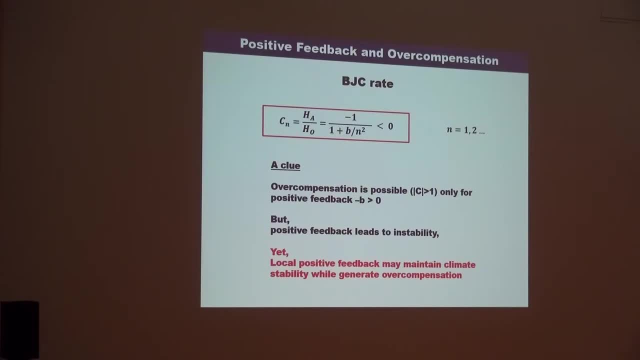 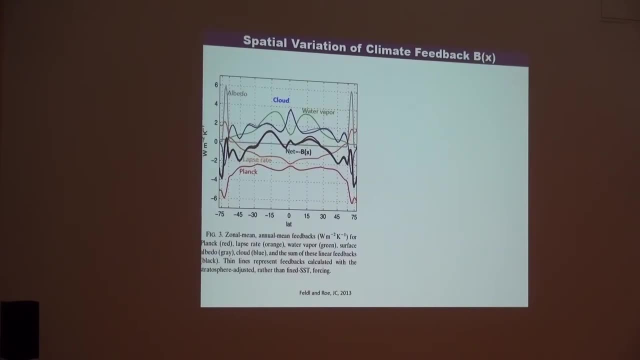 So we are stable? we are not, But it is perfectly possible. locally you may have positive feedback okay, While global maintain it. Well, this is the feedback analyzed from fully coupled GCM. Look at the black line. 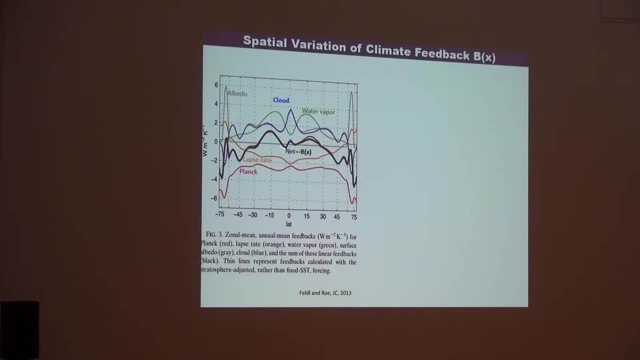 That's the total feedback. at different latitude In the tropics they tend to have positive feedback. High latitude: negative feedback. As a result, the global climate is stable, okay, And this is the CMAP. This is the IPCC model. 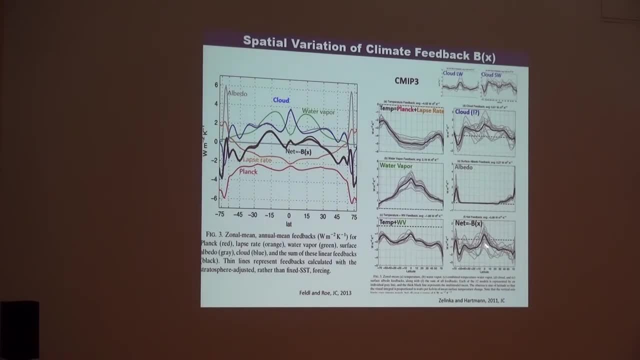 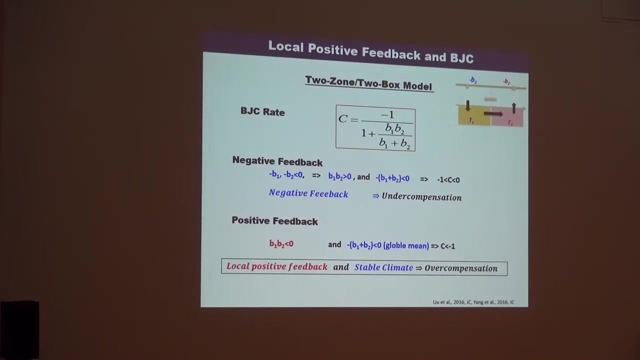 You do the analysis. just look at this file: Final net feedback: Tropics positive feedback And the extra tropics negative feedback. okay, My point is that you could have positive feedback locally in a stable climate system. Now the next minimum model to do this: 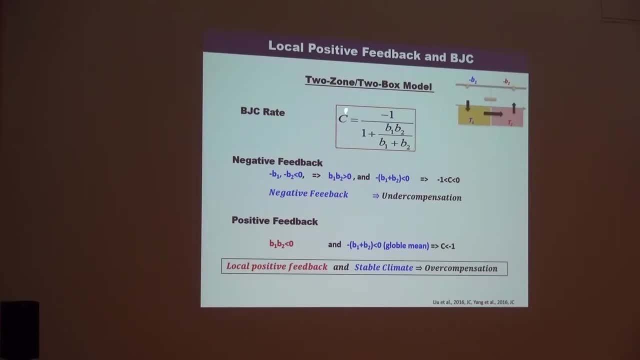 is you make the two box or two region, You can still derive the equation okay. So now you see that if B1, B2 is local feedback in the two region, tropics and the high latitude, if they're in the same direction, 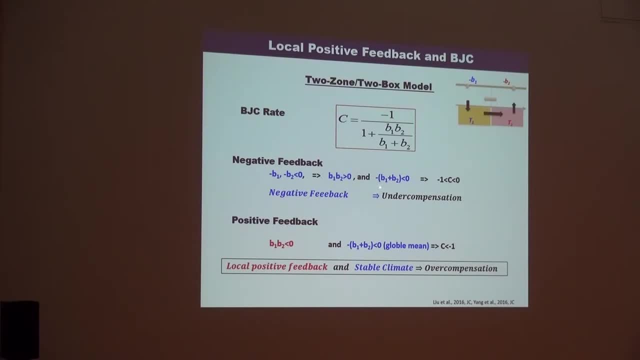 B1, B2 in the same direction. okay, then it has to be. this has to be smaller than one. so therefore the magnitude, so that is under compensation we talk about. But if they are opposite side, so if one of them is positive feedback, okay. 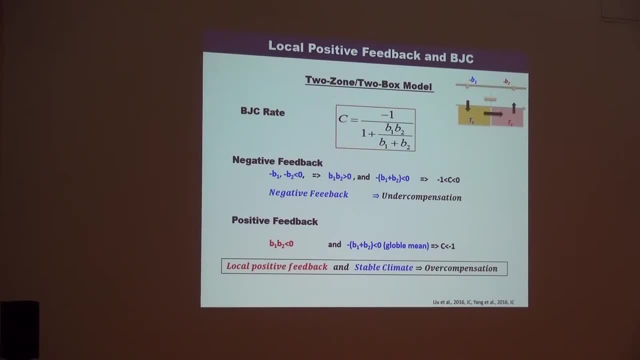 then I can indeed have this larger than one mean value. Okay, you can have over compensation And you can show that in this system, As long as B1 plus B2 is smaller than zero, the system is basically stable. You can solve the eigenvalue stable. 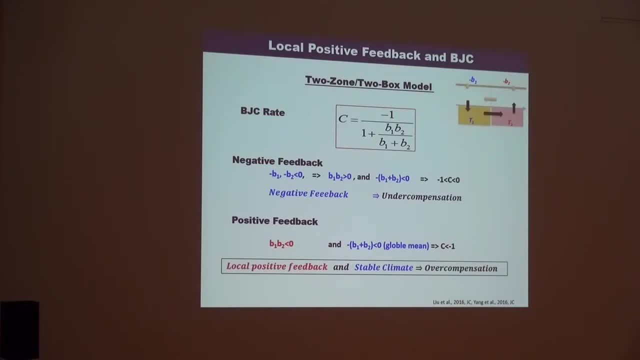 So it's like a global mean. As long global mean feedback is positive, my system- global mean feedback is negative- is stable, But I can have locally. I can have positive feedback okay. So this shows one example, okay. 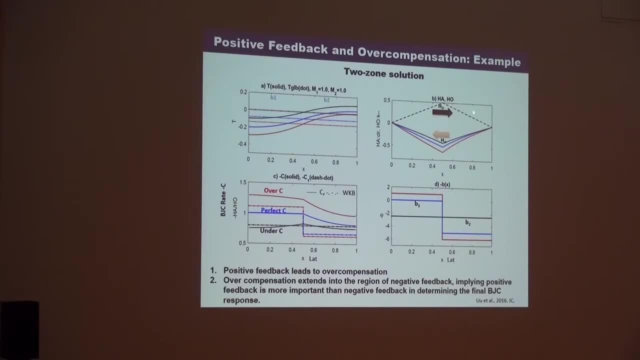 Now in the model I have two region. I still prescribe the ocean heat transport this way. I want to watch What's atmosphere heat transport. In my first case it's like I did before. I have a constant feedback. They are negative, negative here. 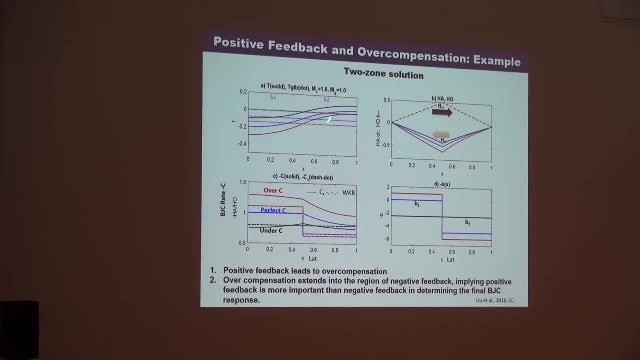 So of course there's a compensation ratio. So you produce, you want high latitude, cold tropics. Therefore the compensation ratio- black- is smaller than one. So that's under compensation we just talked about before. Now watch here. 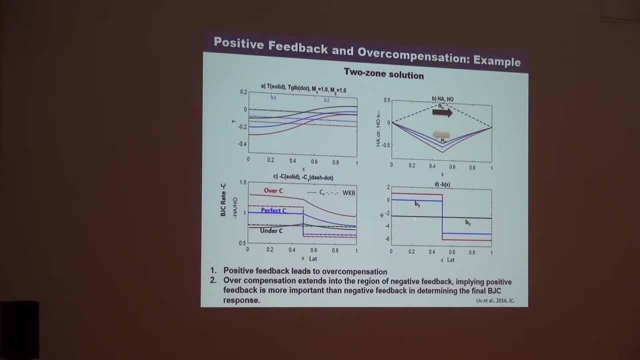 I have global feedback remain the same, But I increase here, but I change this From negative to zero Here, from negative two to even more negative. So global mean the same, But look at the response now. Now, because B equals zero here. 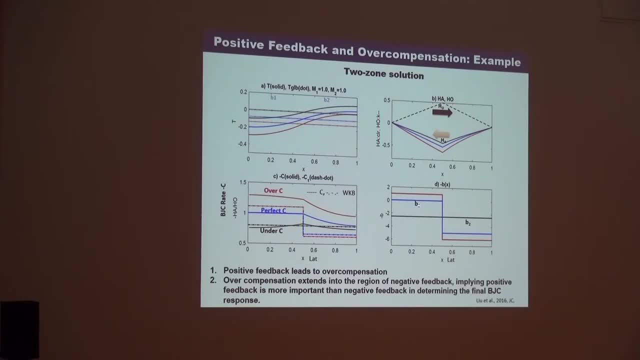 So here is perfect compensation, Because locally in the tropics here there's no energy going out, So whatever come in has to go out. The perfect compensation. okay, And you further helped in this region. Even though it's more negative, it still helped to make them. 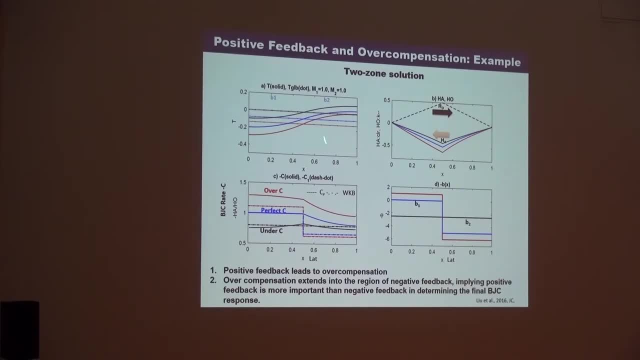 towards a higher, which is ratio. Look at further. If I now increase this to a little bit positive in the tropics, But high latitude making more negative, So global mean the same. Now you can see here You start to have over compensation in this region of local positive feedback. 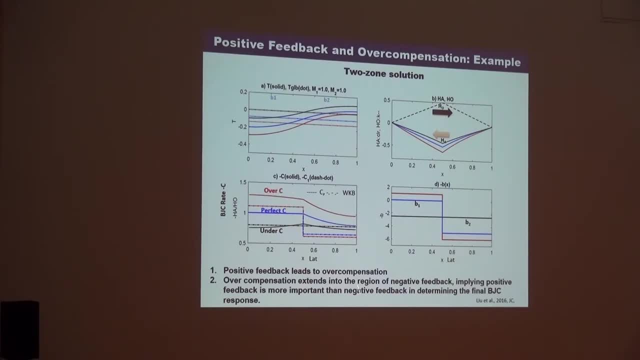 And that will even spread into other region, Even though here actually it's more negative feedback. Now one feature: you see that if I have uniform feedback, it's warm pool, cold response. So you can see that. You can see that. 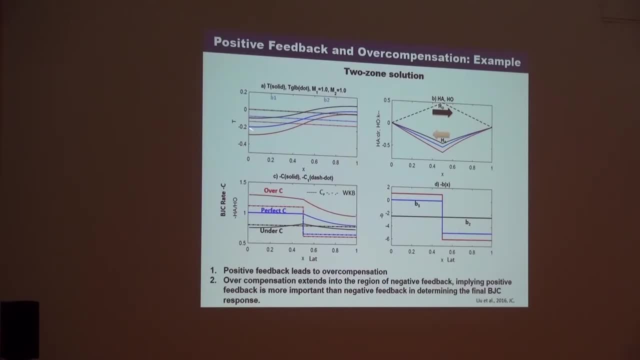 It's like cold response, It's like bipolar response, but global mean remain more or less the same. But when you have the positive feedback locally, the global mean temperature is also changing. Not only as the gradient, global mean temperature is also changing. okay. 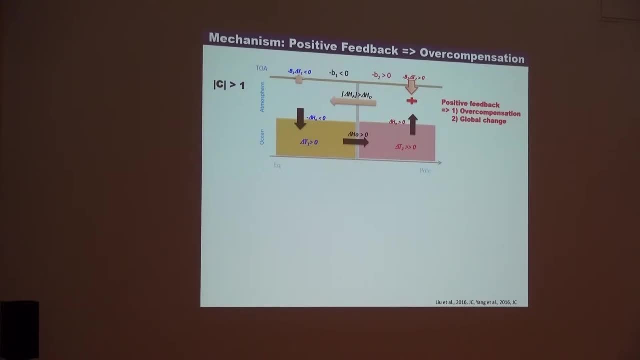 Why is that? Let's again think about this simple model. Let's do the experiment- salt experiment again. We transport heat. this way, Heat comes out. That's the same. Now, the difference is that this is a positive feedback. 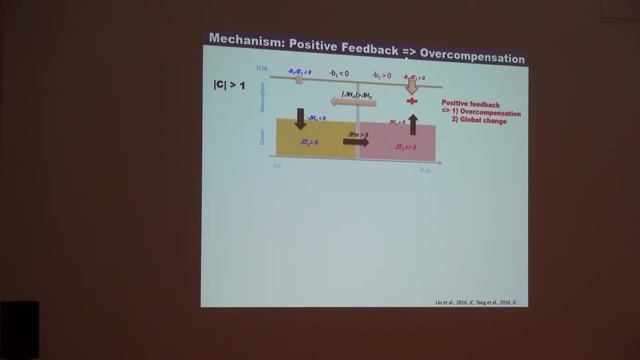 What does it mean? positive feedback. I have one watts per square meter heat come here. I have additional heat come in because of positive feedback. Okay, Now, if that's the case, what else the atmosphere, heat, transport go? The only way is go back here. 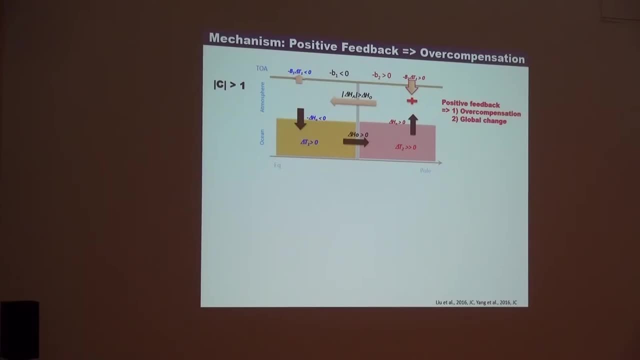 So you have this come in this additional, So you have more heat transport back than what you prescribed at the beginning by the ocean heat transport. So that's why the local positive feedback matters. Okay. And the other thing: you can see that because in this region it's supposed to be warmed. 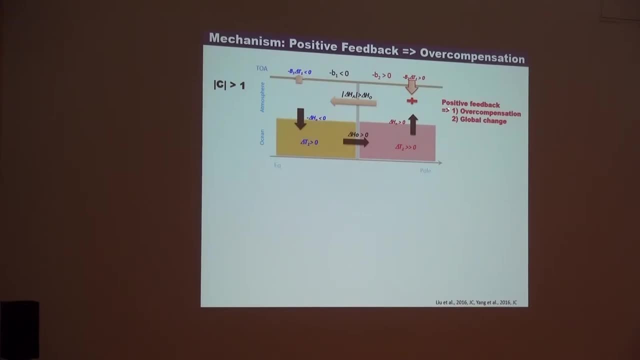 up and then you have positive feedback so you generate lots of heat. This transport back so you produce global warming. This here: originally you lost some heat, You want to be cooling, but because you suddenly generate extra heat from here, so you can. 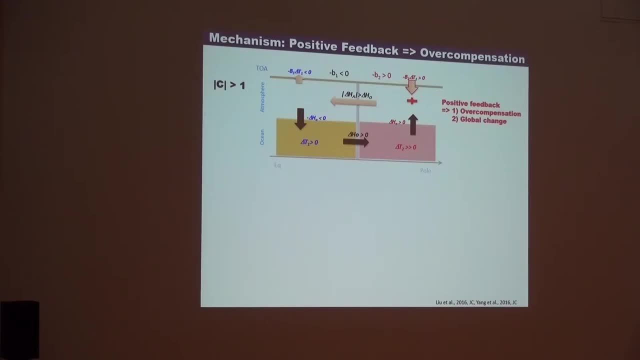 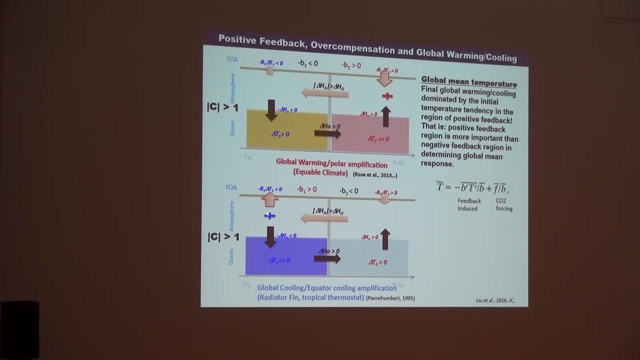 still warm it up, So the entire globe will be warmed up. if the downstream of ocean heat transport is increased is positive. Okay. You can have the opposite direction. If the upstream heat transport is positive feedback, then it's global cooling, because 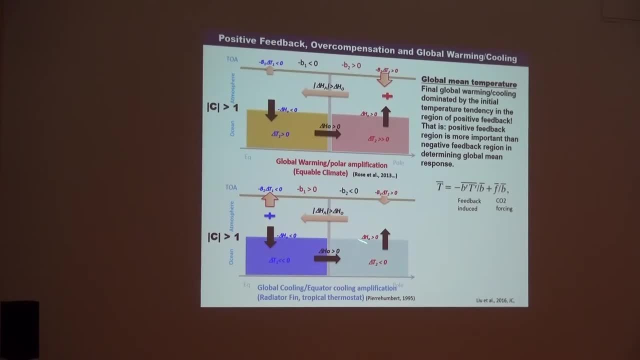 you pull heat away, you lose heat, but you lose more heat. then this is spread around. you got an extra compensation, but it's global cooling, Okay. So the point is that when you have local positive feedback, you can indeed generate. 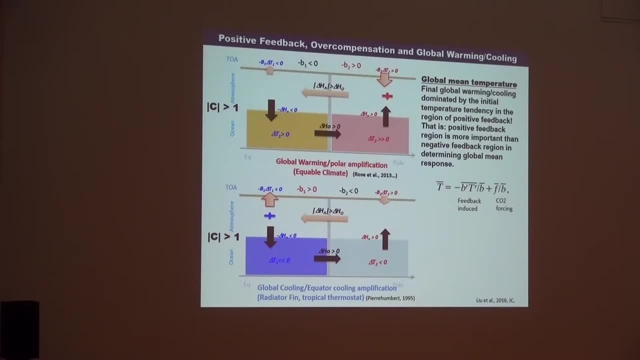 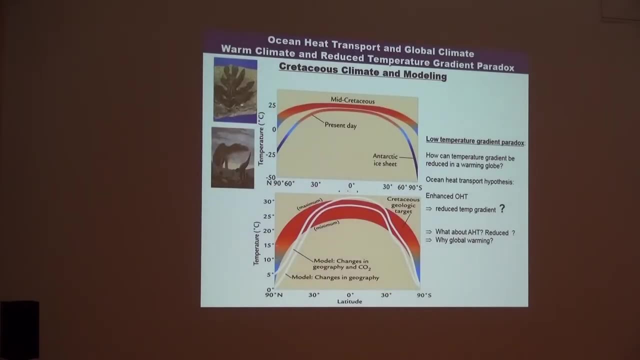 over compensation And, in the meantime, global cooling. Okay, So the point is that when you have local positive feedback, you can indeed generate over compensation And, in the meantime, global temperature change, global mean temperature change. Okay, This might have some implications for some paleoclimates. 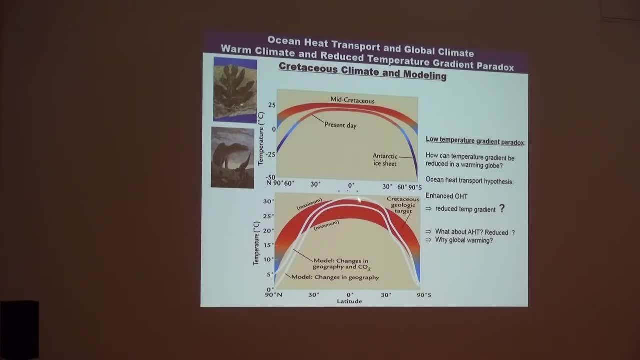 For example in Cretaceous. you know, there is always one puzzle why the current model couldn't produce this reduced gradient. One hypothesis: the global mean temperature is warm. One hypothesis is that the ocean heat transport increased. But if ocean heat transport increased, if the feedback? there's no positive feedback? 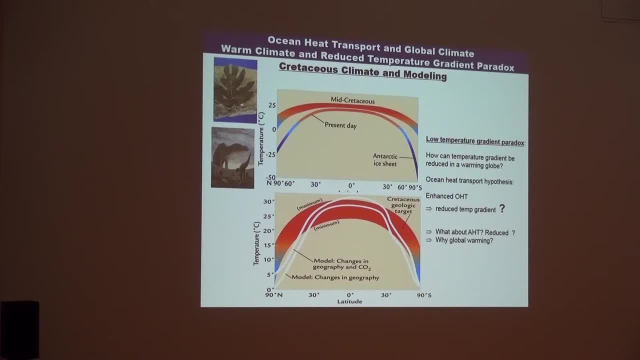 you just simply reduce the gradient, You don't increase global temperature. Okay. So what you need if ocean heat transport is increased is responsible for this. the additional thing you need is to have additional positive feedback at high latitude Clouds, whatever. 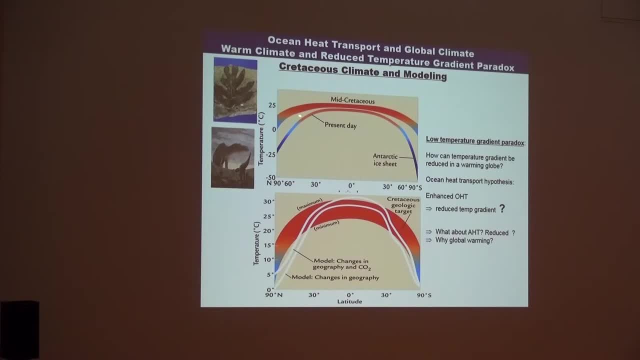 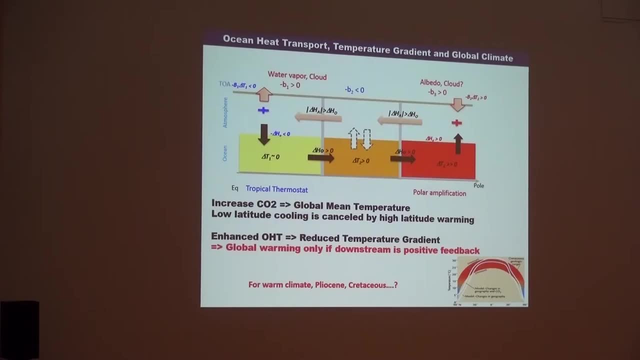 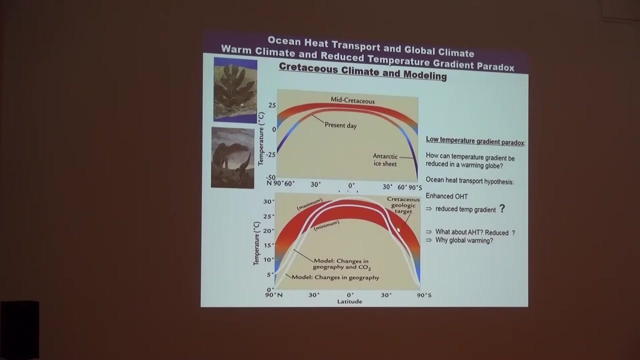 You know some people talk about equal climate. Have positive feedback, Then that will reduce gradient, increase global temperature. Okay, Yeah, Yeah, In polar amplification in the, in the current global warming case, current global warming. 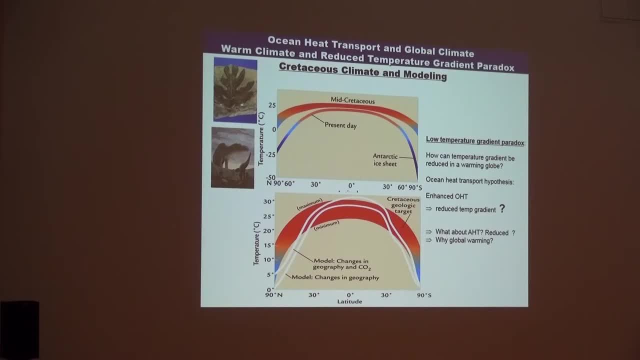 case- I will talk about it later. It's mostly actually you can have compensation And the global mean temperature. you have some change, not so dramatic in this case. This point, my point, This is different from the current global warming. 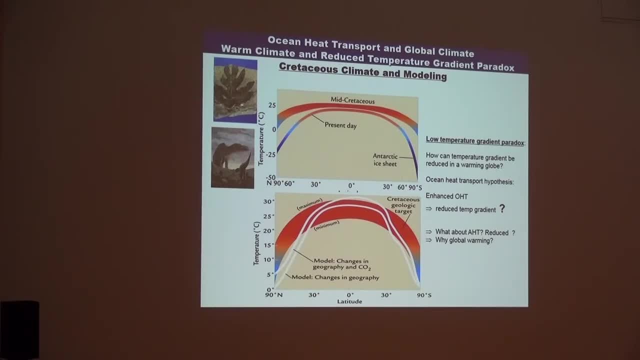 is that because you have radiative forcing? This is, if the forcing is by ocean heat transport alone, Let's suppose radiation, no change, okay, Just to transport heat. If you have no positive feedback, the only thing you do is you warm it up. 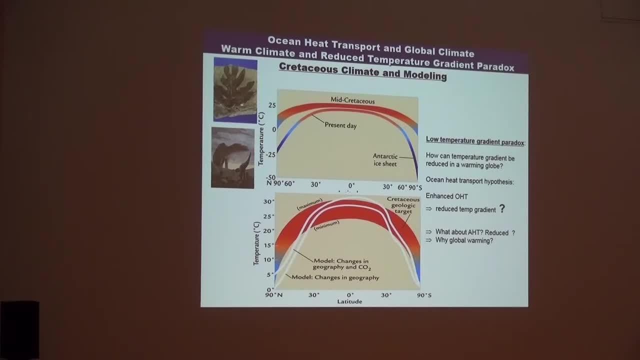 you cool this. no global temperature change. How do you warm up entire globe? Then you need in the region downstream you also have positive feedback, Let's say cloud or some property change. Then it's like you generate, mysteriously generate additional heat, right. 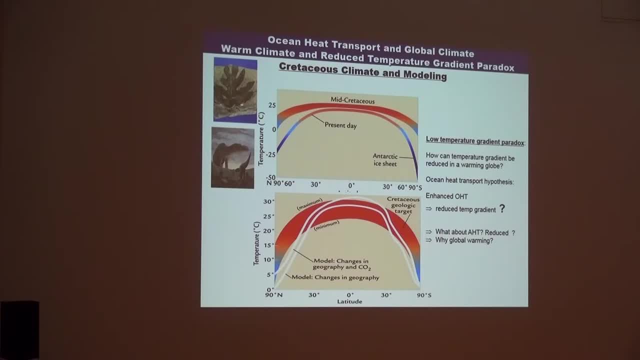 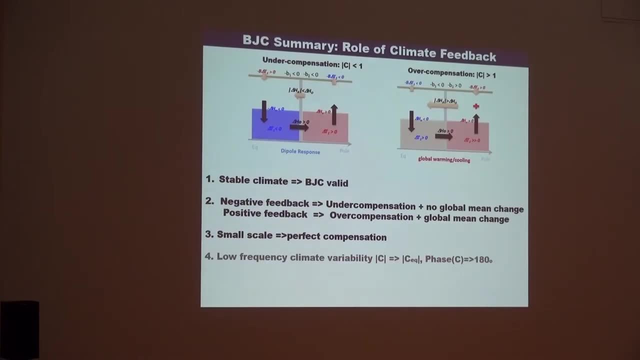 Because there's a positive feedback, Then it's redistributed back so it can warm up the entire globe. So that's the point of this, of this, okay, So for this part, the summary is that as long as the climate is stable, global mean is stable. 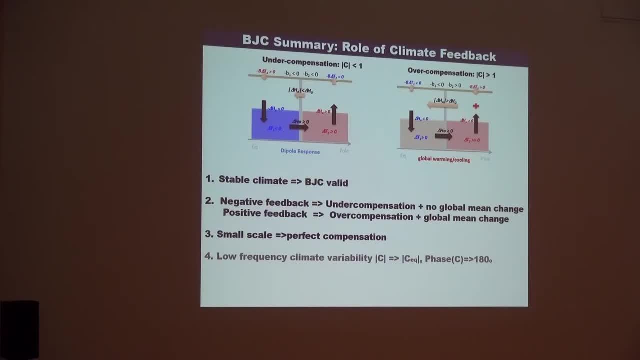 that biogas compensation is always valid if it's caused by the ocean heat transport. The second: if the next feedback, then it's so-called under compensation. You transport one watt 0.7 coming back, But if you have a local positive feedback, 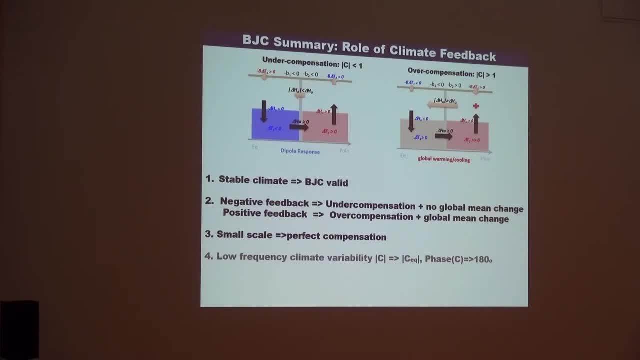 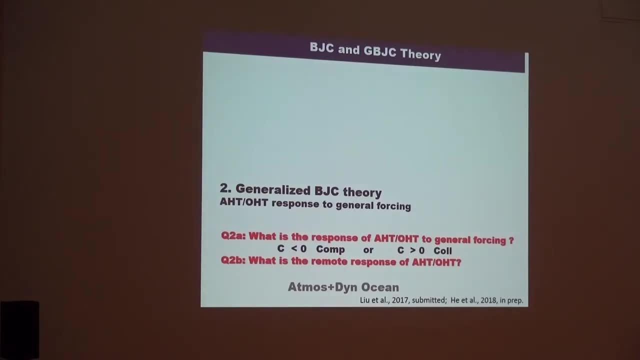 you could have over compensation One watt, I can have 1.2, okay And global mean temperature change, And there are some other minor features I'm not gonna deal with. So now let's go even further to the generalized theory. 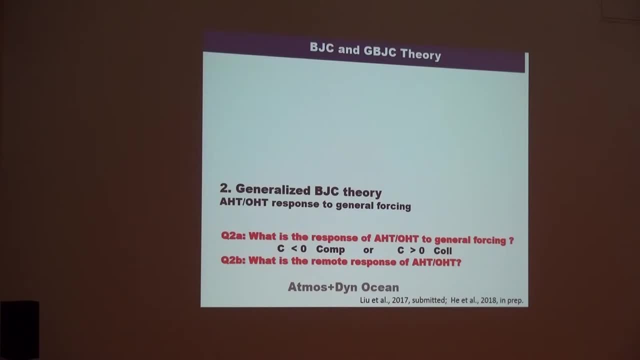 okay, generalized biogas compensation theory. See, here's the question. I can have a general forcing. It doesn't have the ocean transport, Maybe greenhouse, maybe solar insulation, Maybe some whatever volcano, whatever. In this case, I perturb the climate. 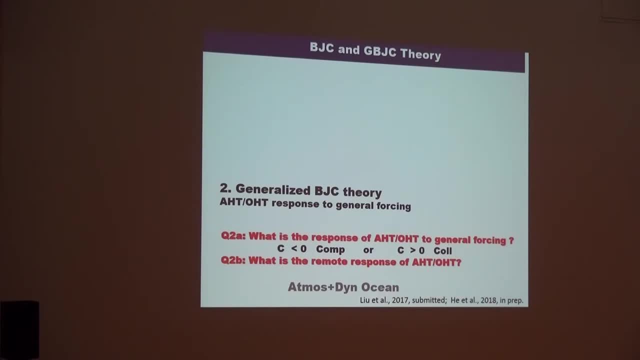 How is the atmosphere ocean heat transport respond? Okay, my first part is that you notice that I only perturb ocean. then see what the atmosphere response Okay. but now I'm doing more general case. This is some global warming response. 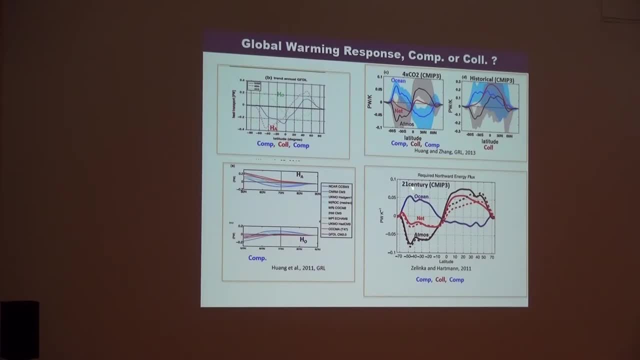 Different models show the global warming. Some case you do see opposite. You know most of case opposite response here, Although in the tropical region, here you see they tend to go the same direction. okay, Some here tend to go the same direction. 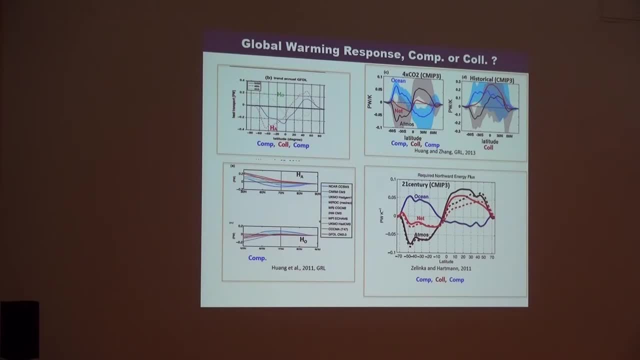 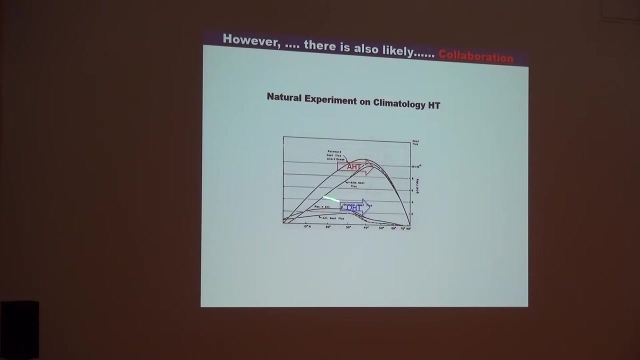 So in this global warming case it's not very obvious. You know, sometimes you have compensation, Sometimes they may not. That's what the model says here. Now we know, as I said, this is a natural example. When you have a solar radiation, come in. 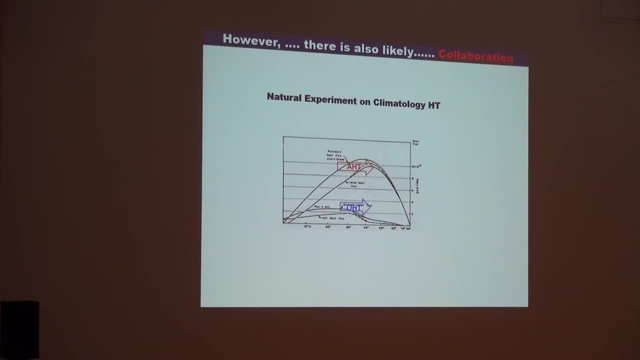 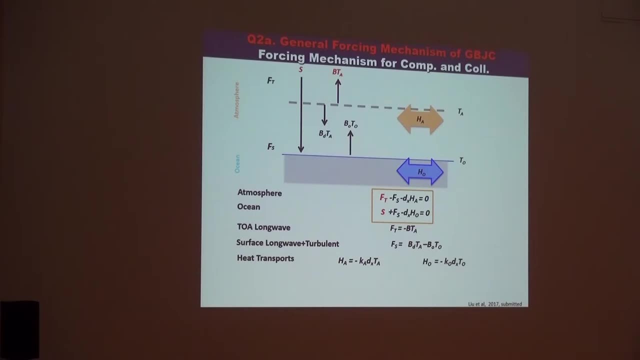 they tend to go. just go to the polar region. It's a collaboration response. How do we think about this? Now, this: we have to increase the model complexity a little bit. Instead of using a slab ocean, I have to in the ocean. 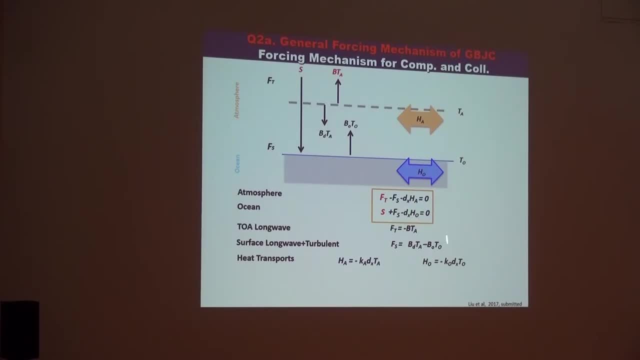 also add heat transport, which I can parameterize similarly as diffusion of the temperature across the ocean. So it becomes a two layer model And I was stuck on this for a while before I realized that actually it's a very simple problem, Because think about it. 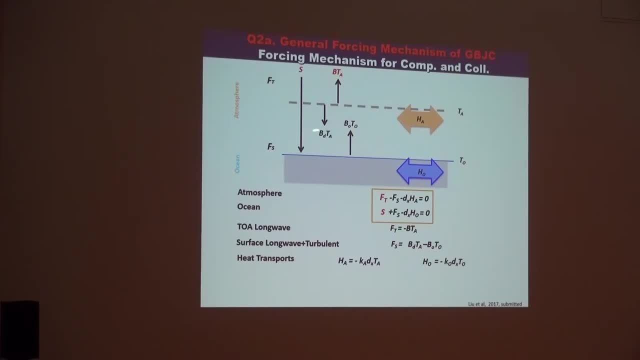 Let's think about this: Fs, This is surface heat flux, Surface heat flux change between: If I have surface heat flux change. look at the equation here. It's zero sum game. I give to the atmosphere, I lose heat. So to the ocean and the atmosphere. 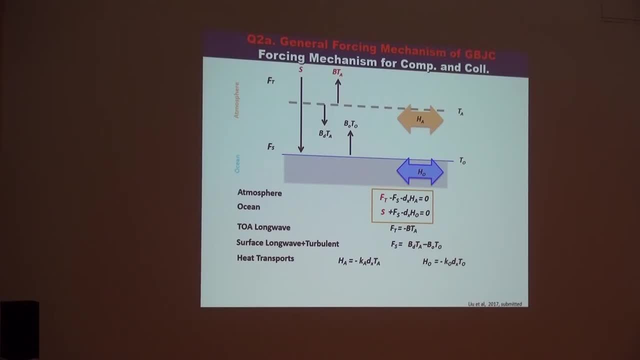 the surface heat flux is opposite sign, So the response has to be opposite. So they should produce opposite compensation response. That goes the same to ocean heat transport. In the steady state, when you have ocean heat transport, there's nothing, nowhere else to go. 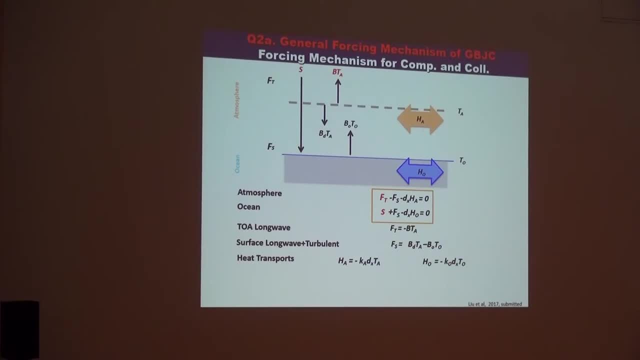 You have to produce changing surface heat flux. Therefore, you have to have compensation response. That's the case we discussed earlier. When you have ocean heat transport response, it's always compensated. okay, Now, that is so. it says that if I perturb surface heat flux, 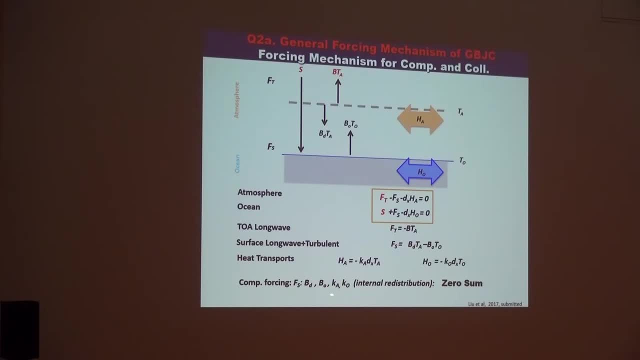 okay, I have compensation response because zero sum game, One game, one lose it's opposite response. However, from this point of view, you think about this: If I have solar radiation, come in. well, that's a one-way situation. 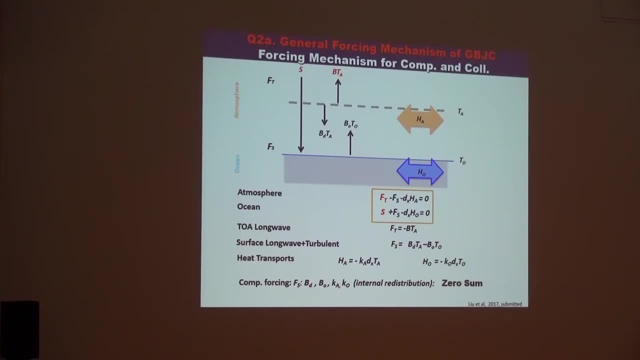 I got heat in both atmosphere, ocean. We don't have to fight, Let's just happily share them. you know, go the same direction. So in that perspective, if I have solar radiation I should produce a collaboration response. Same for the top of the atmosphere. 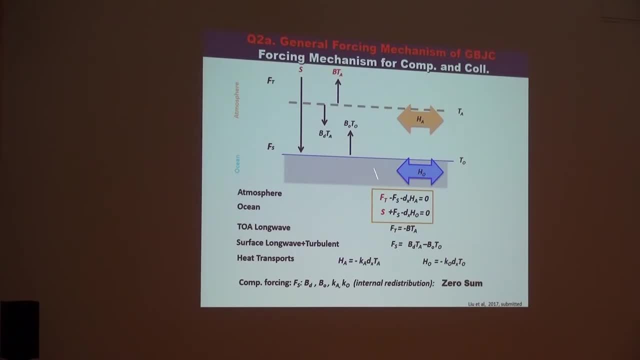 If I have some perturbation only in the top atmosphere, then that's the same for both- atmosphere, ocean. There's no fighting between them, So it's a win-win situation. Both have to go the same direction. So before going to the mathematics trying to solve this, 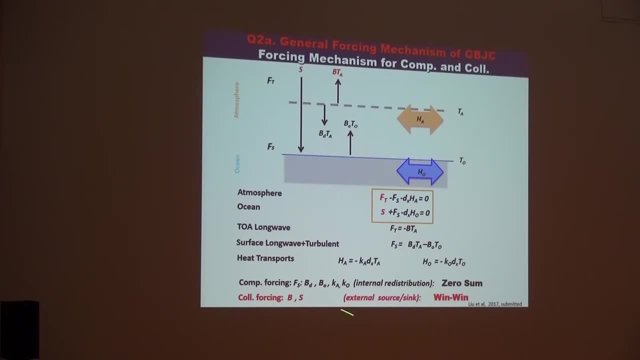 we can think about this physically. If I perturb any parameter that results in surface heat flux change, I should produce compensation response. On the other hand, if I perturb top of the atmosphere, it's external forcing. then I got a win-win situation. 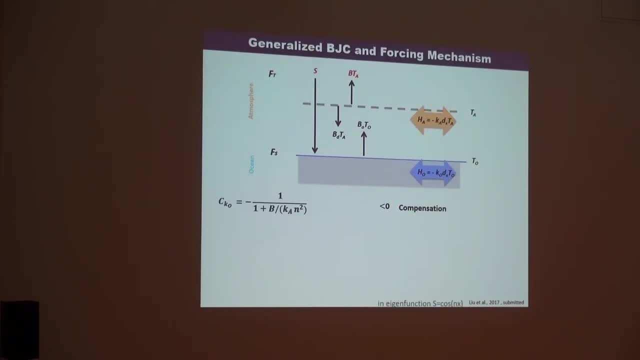 This should go to collaboration response And that's exactly what happened in the mathematics solution. You can solve this again in the eigenfunction cosine V comma analytical solution. You can find that the compensation ratio, if I only perturb this ocean heat transport coefficient. 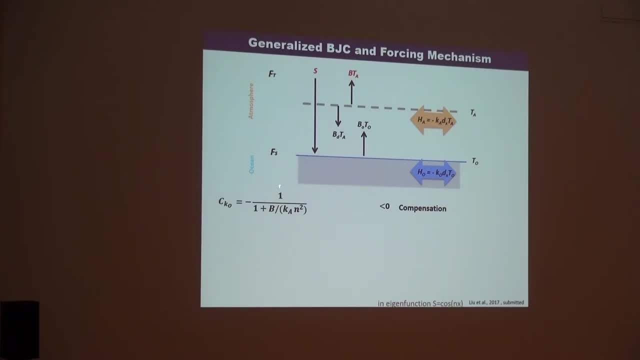 that is, if I only perturb ocean heat transport. the compensation ratio: this form is very similar to what we just talked about before. It's a one one, then divide by this B here, So it's a negative, so it's compensation response. 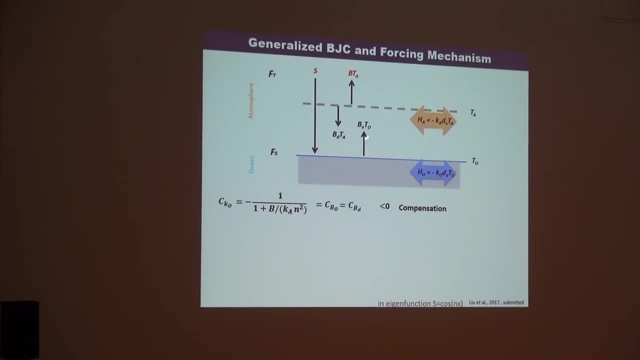 Now I didn't expect, if I perturb other parameters here- so they all perturb surface heat flux- they produce quantitatively exactly the same compensation ratio. I was thinking they would be sort of more or less negative compensation, but I didn't realize they are actually. 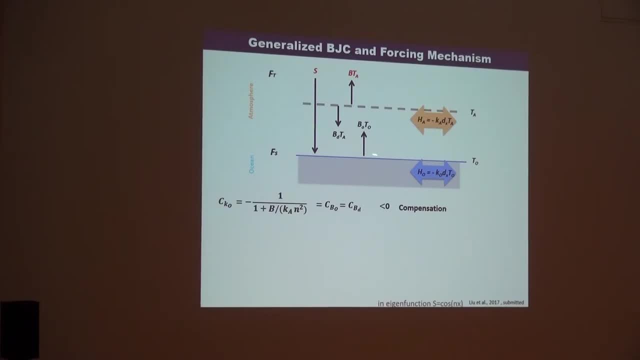 exactly the same compensation. So it just shows that if you perturb surface heat flux, they are just the same same response compensation. And if I perturb top of the atmosphere, yes, they are indeed positive collaboration response. That was expected. 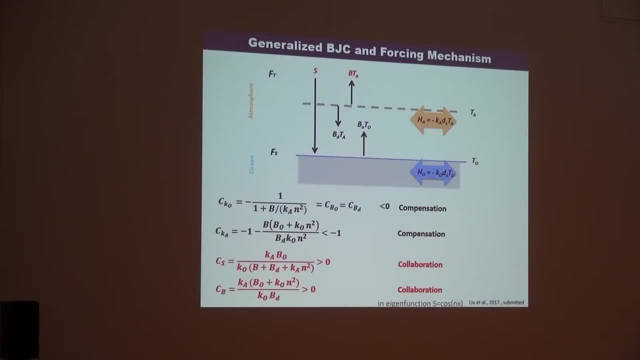 So now actually, this part of the problem becomes actually very simple, right? It just depends on what perturbation forcing. If you perturb predominantly on surface heat flux, then atmosphere again, ocean loose, or vice versa, then the response is opposite. 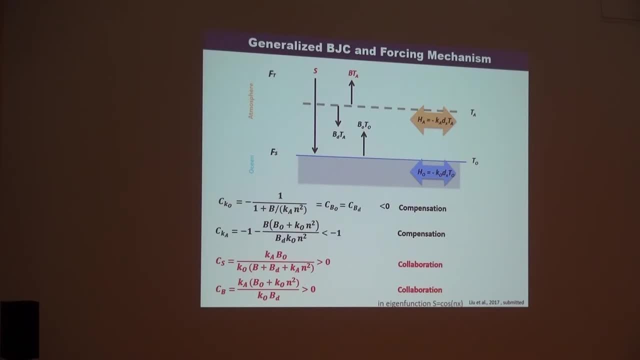 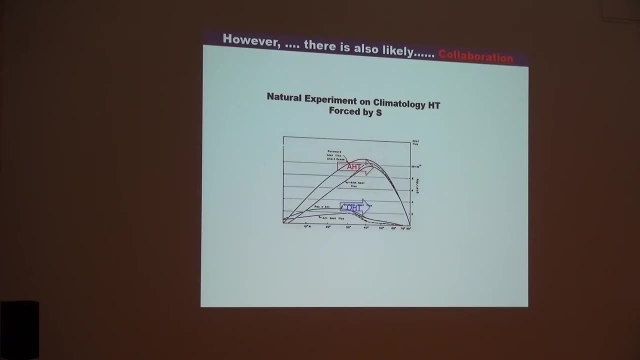 That's compensation response. If you perturb a top of the atmosphere or shortwave, then it's a one-wing situation, then it's collaboration response. okay, So the shortwave response, that's obvious, because you have the shortwave response. 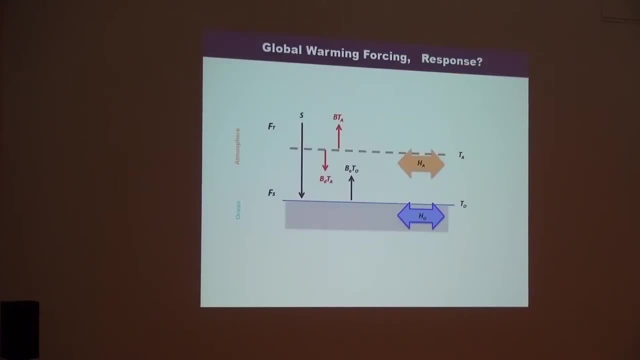 shortwave forcing. that's collaboration response. Now we have to be a little bit careful now on global warming case. The case of global warming is that it increase CO2.. Therefore, the longwave radiation increase toward both the top and the bottom. okay, 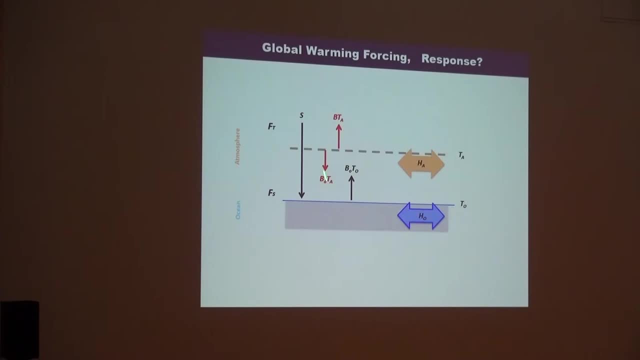 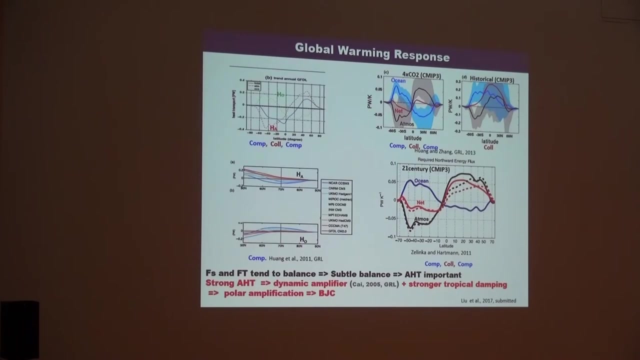 Now, this one will give you collaboration response. This one will give you compensation response. So it's actually not obvious: to a global warming response you have to have compensation or collaboration. okay, from this perspective. So anyway, I did go to. 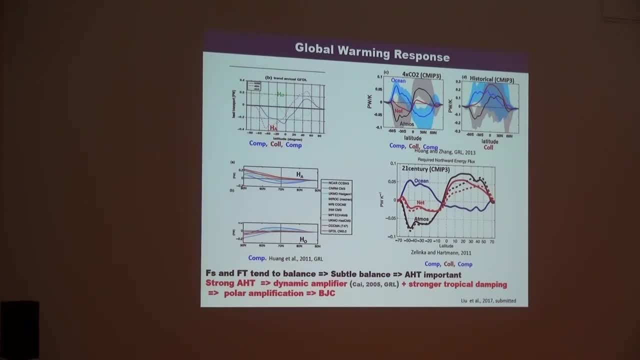 of the theory, saying that I'm not going to show that In the global warming case you have to go to secondary factors. The first order they sort of canceled out, You have to go to secondary. okay, The spatial distribution of the coupled feedback. 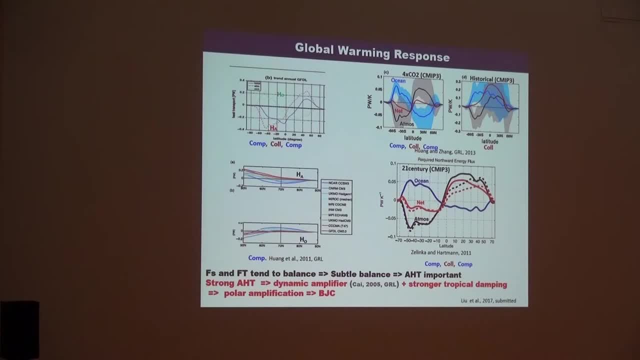 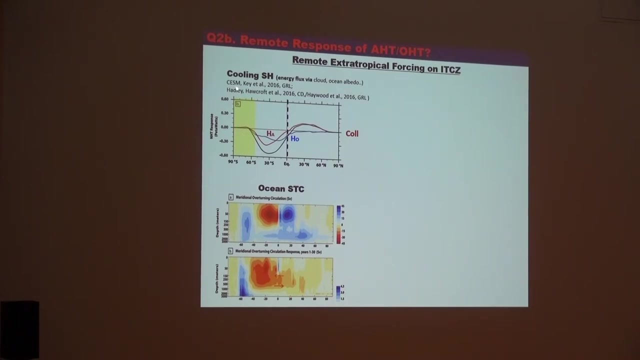 become actually interesting factor. So you need atmosphere, transport heat toward the north, but in the meantime you also need a stronger damping in the tropics to make compensation response. Now, final question: As I showed you, this GCM results, I perturb clouds in the south ocean. 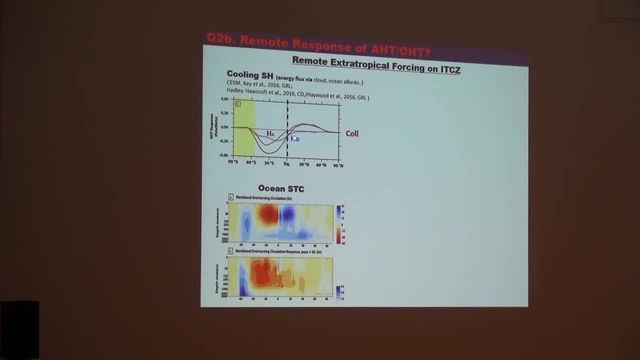 My heat transport is always same direction and have very little response when you go here And when they analyze the coupled system. yes, it is hardly circulation, subtropical cell change And this seem like it's not give you a very strong heat transport response downstream. 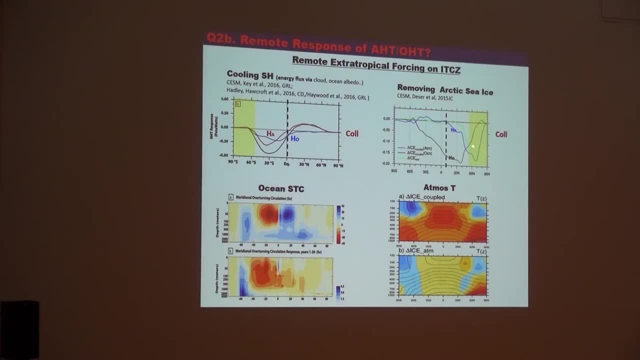 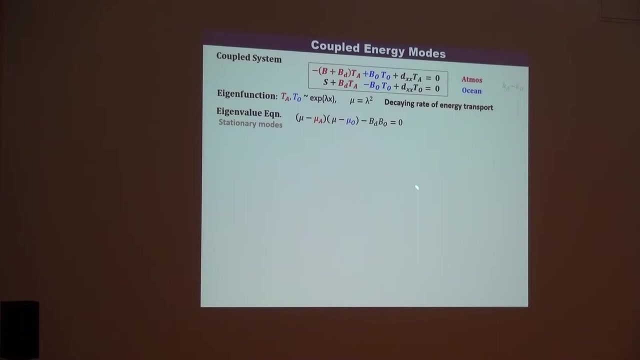 Same thing for this. When you perturb arctic sea ice and the ocean atmosphere, heat transport can go the same direction, not opposite. That is what people think the ITCZ want to go. Well, let's think about this. This problem can be thought as actually coupled mode. 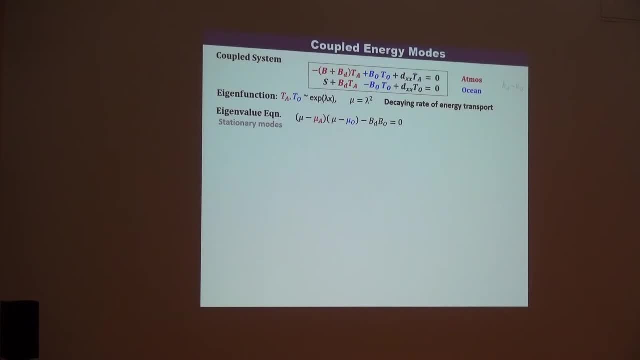 It's like wave radiation. When I talk, you hear right? That's because sound wave radiate to your ear. Here is the same, except now the wave is not the normal wave. It's not even a raspy wave, It's really some kind of energy coupled mode. okay, 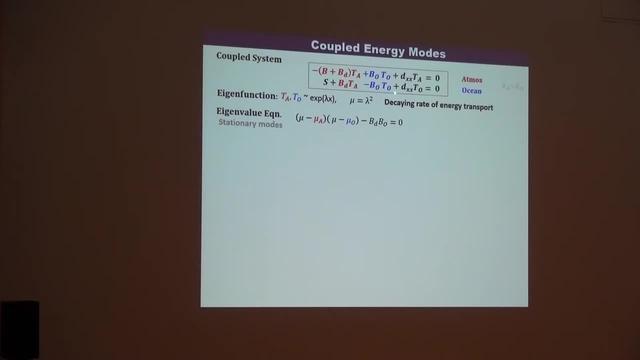 You have DXX here in the atmosphere, in the ocean, here. So you've got an atmosphere. it's diffusive but it's stationary. you know, For wave you should have a partial T here, but we're talking about stationary wave very long time. 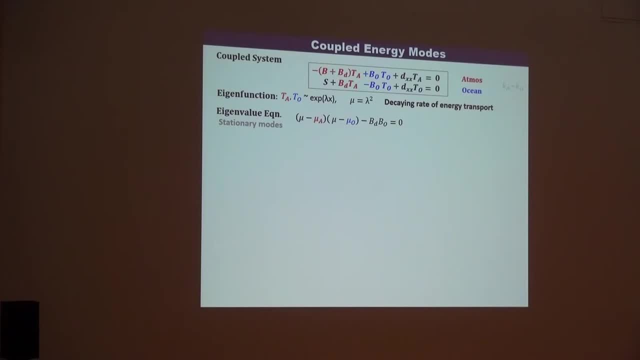 So in this kind of stationary wave really the damping becomes scale in the spatial scale instead of in time damping. because you fix time. time becomes zero. So the only thing can change is space. The space become damped. response: okay, 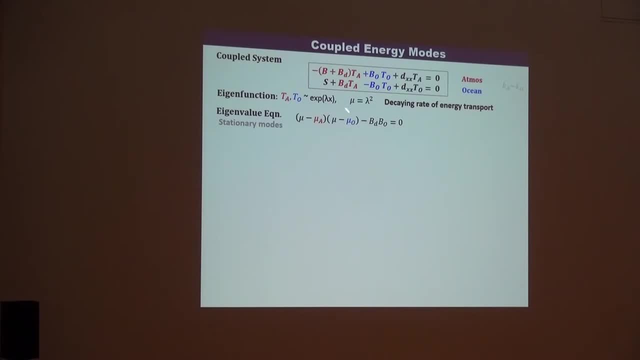 Now you can solve the eigenvalue in the damping scale. the damping scale here eigenvalue, And there is one eigenvalue just for the atmosphere. that is, if I only have atmosphere, I should have this damping, because radiation have damping. 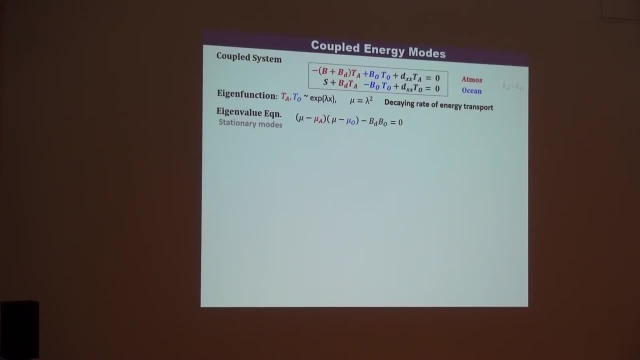 There's another one for ocean damping, only for ocean damping. So now let's think about the coupled system, The simplest case: if I have no coupling, if I have no coupling in this system, if I have no coupling, you can solve this. 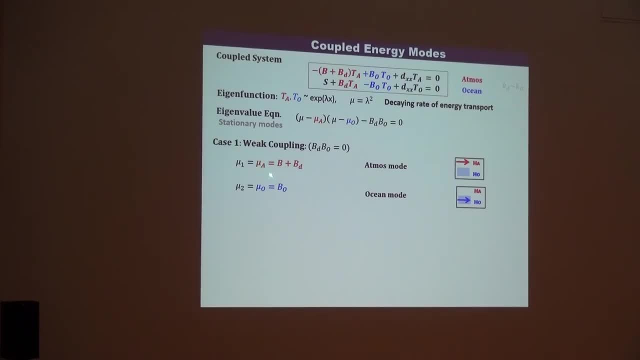 You have two modes. One mode has exactly the atmosphere damping rate, In this case, atmosphere transport heat, no ocean response. okay. The other mode is pure ocean damping rate. Ocean transport heat, atmosphere has no response. It just because there's no coupling. 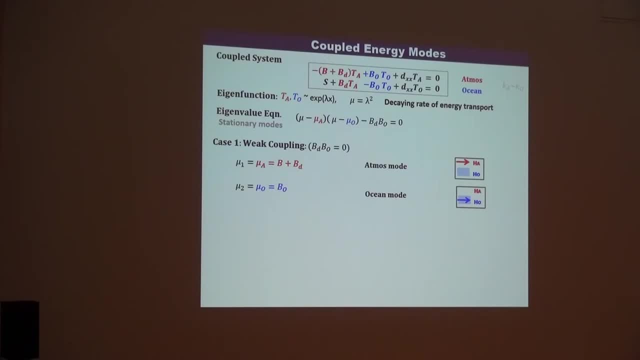 the two just go, you know, independent. So this is kind of a simple case. but our real world, if you calculate regime, it's actually in the opposite case. It's a coupling much stronger than the top atmosphere radiation. 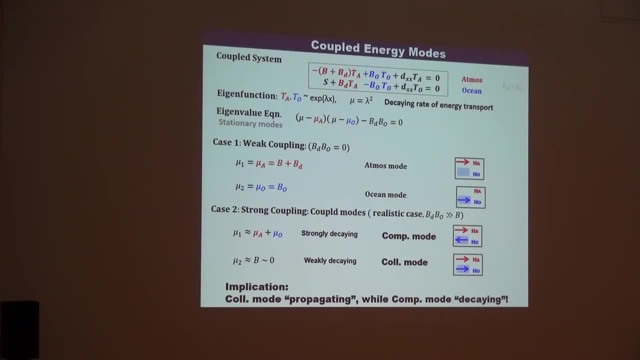 Because this radiation, especially surface heat flux, then when you actually include a turbulent heat flux, that's very strong. okay, It's almost five times larger than the top atmosphere pure long wave radiation. So the realistic regime is this: much larger than this. 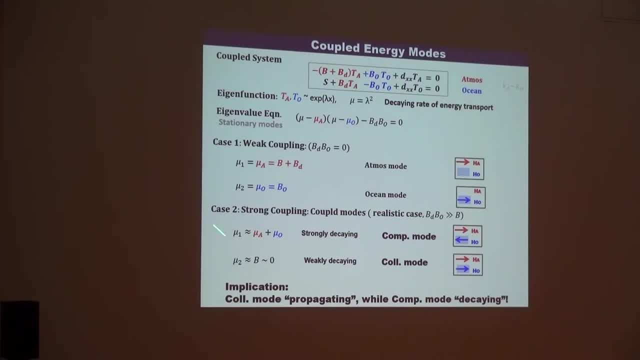 So this is very big. Coupling is very strong, In this case the coupled mode. you can solve this interestingly. One mode: the damping rate is atmosphere damping plus ocean damping, So this is a heavily damped mode. okay. 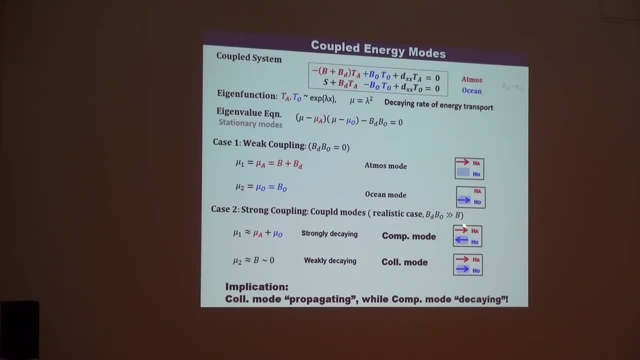 It's two together Also interesting. you look at the eigenfunction structure: Atmosphere, ocean- they're always opposite. So this mode is compensation response, but heavily damped. The other mode is very, very weakly damped. 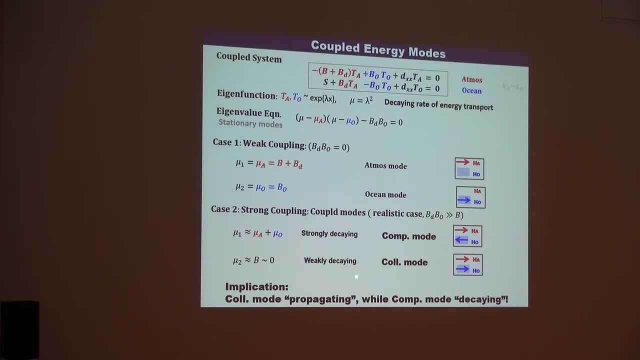 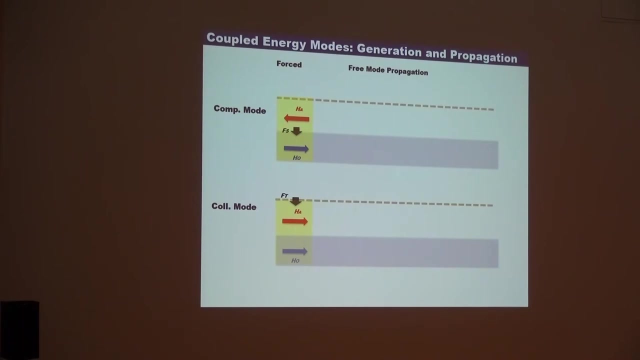 just the top atmosphere Radiation very weakly damped. Now, in this case, the eigenfunction structure, they are in the collaboration response. okay, So what this tell us is that in the coupled system we have two coupled energy propagation modes. 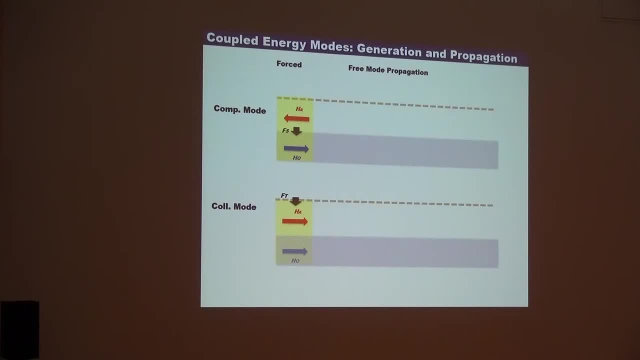 This is not a raspberry wave, not like that. It's just energy coupled modes. One mode, compensation mode. For example, I can excite by surface heat flux, then we can have compensation. we talk about How it's propagating. 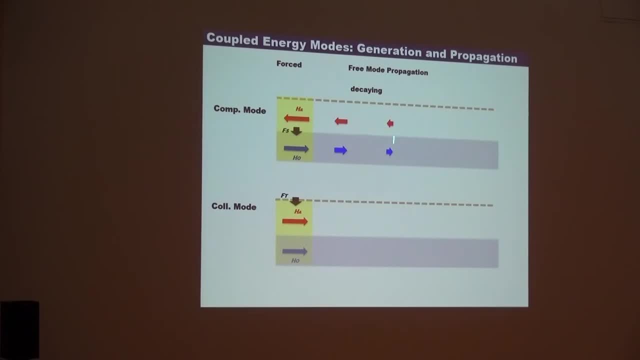 Very slowly, opposite direction, quickly damped. The other mode, let's say this one suppose I use top of atmosphere, I produce collaboration response. They probably quickly and very little damp. they can propagate far away. okay, And so because the collaboration mode 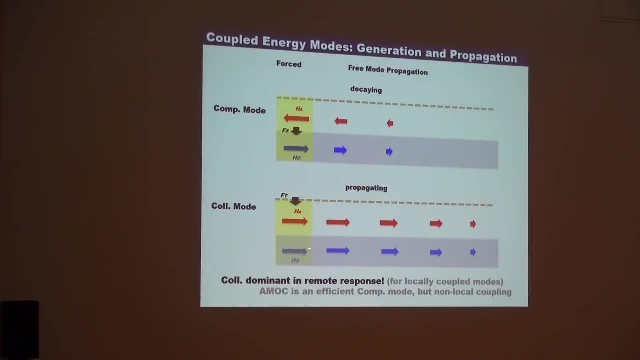 has very little damping. so if I have a force in here, the far region response should be dominant by the collaboration mode, not by compensation mode. Compensation mode is damped from the region of forcing. okay, It's sort of like in the climate dynamics. 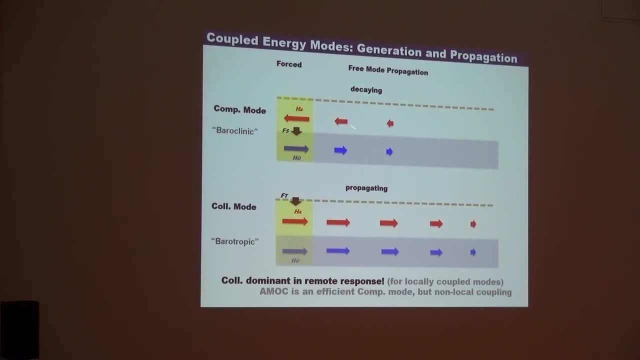 the atmosphere-ocean dynamics. there's one thing called the baroclinic mode, where the upper layer, lower layer, go opposite direction, whereas the barotropic mode they go the same direction, But here it's a completely different physics. 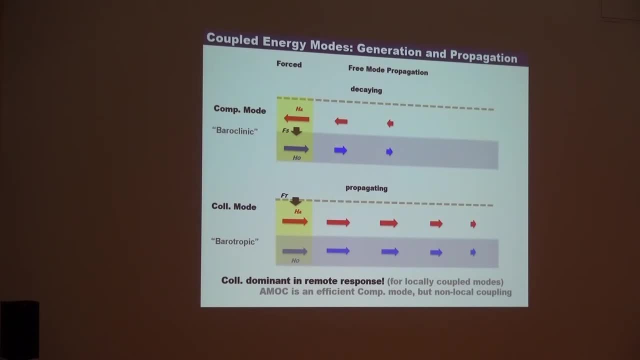 Here's completely different physics. Now you might say: well, this is mathematics, This mode is heavily damped. This mode is not heavily damped? I would say no, it's not, because the physical mechanism is very simple. 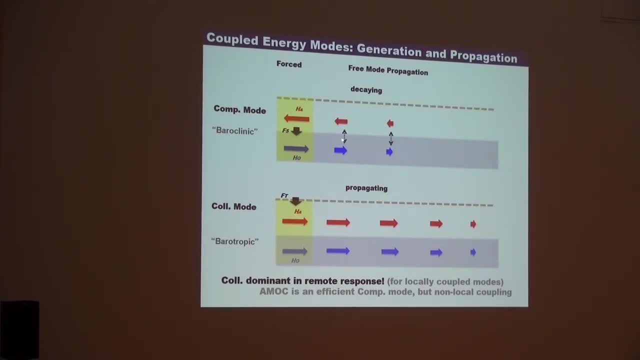 Why the compensation mode damps fast. It's because, as I said, compensation is mostly exciting surface energy, flux. Surface damping is very strong. You have the latent heat, sensible heat, very strong damping, so quickly damped out, While this mode, because they don't involve 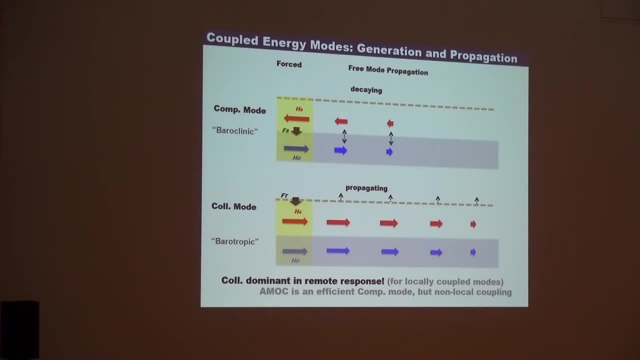 too much surface energy change. It really just top of atmosphere energy change, Very weak damping. so that's just long wave radiation steam and bottom of formula, just very weak damping. okay, At least you know, it's probably 10 to 20% of this okay. 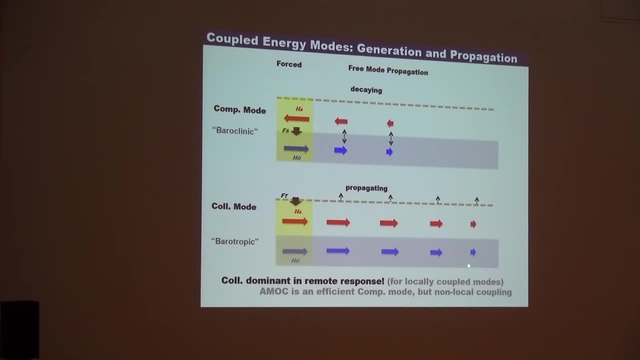 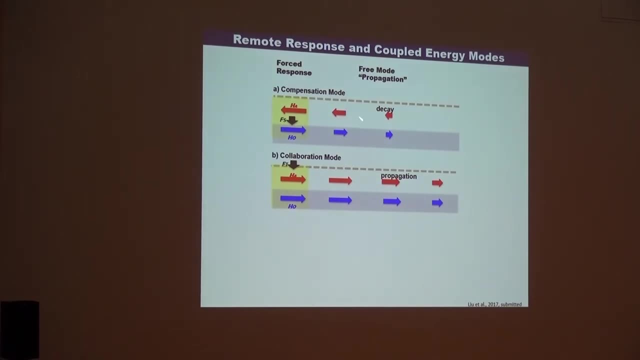 So that's why, physically this mode, it should be less damped, while this mode is heavily damped. So for the remote response we have two kinds of mode, and remote response tend to be dominant by collaboration response, except except this one thing. 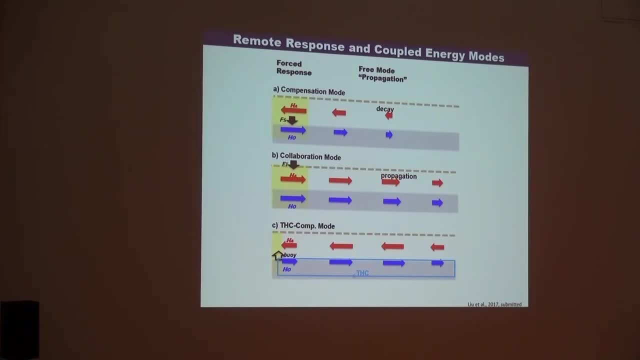 This are all coupled through surface ocean-atmosphere coupling I could have if I perturb Atlantic Meridian Overturning Circulation. they sneak out from deep ocean across entire hemisphere, deep western boundary current all across, so they transport heat. 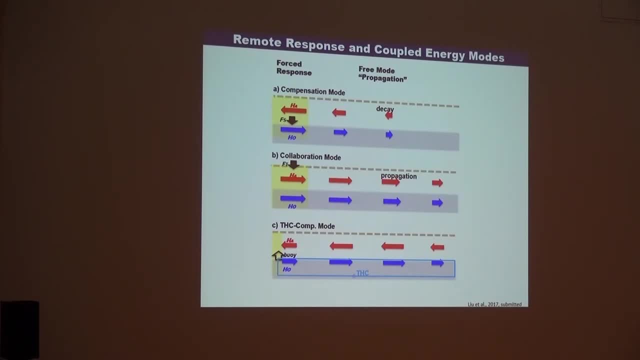 Then they come up. surface heat flux affect atmosphere. Now in this case the remote teleconnection could be very efficient. Now you can indeed produce compensation, just like the first part I said: If you give ocean heat transport, then atmosphere can have compensation. 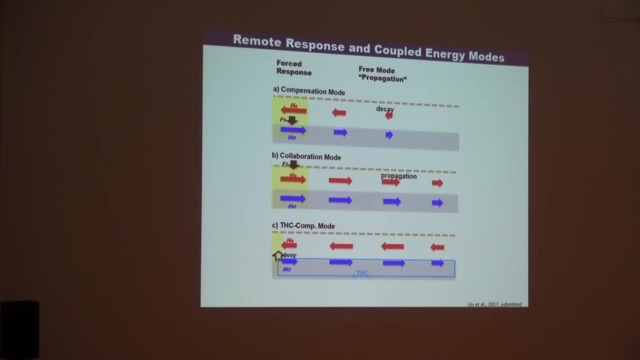 So you can have a very strong compensation response. okay, So the conclusion is that in the coupled system, when you perturb it, if you don't perturb AMOC strongly, then you have to have collaboration response, because the coupled mode is less damped. 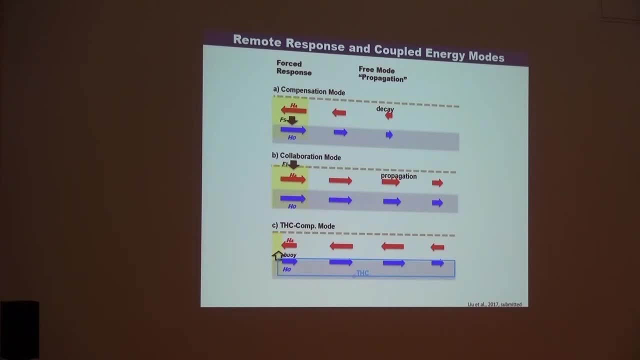 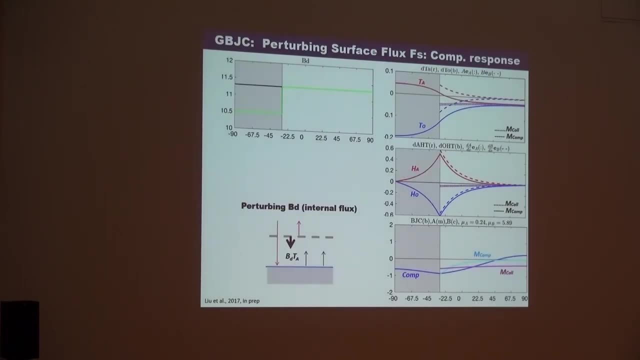 But if you perturb AMOC very strongly, then you can have a compensation response, okay. So it depends on how you perturb it And how much time I have. Yeah, and this just some. I'll just show you one example, okay. 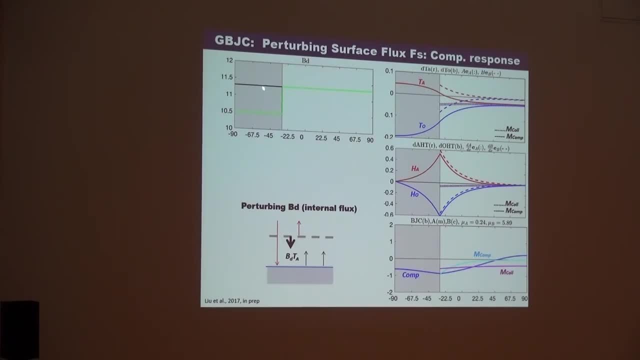 So this in the model, what I do is that I only perturb. I can't remember. yeah, I perturb the surface flux, I perturb this parameter. I suddenly decrease this parameter. okay, Decrease the parameter. 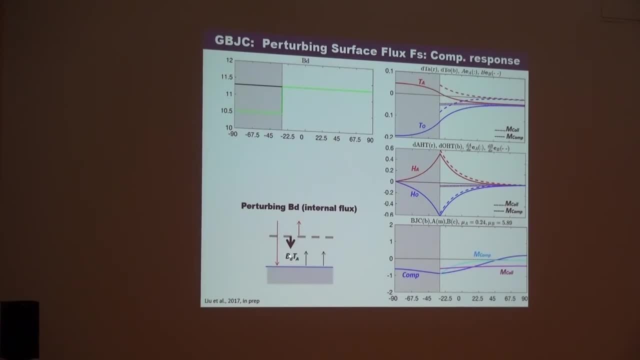 So we know that this perturbed surface heat flux, then it should produce compensation response. Yes, as you can see here my response in this region. that's why forcing region in the south hemisphere region, because I reduce this, so atmosphere. 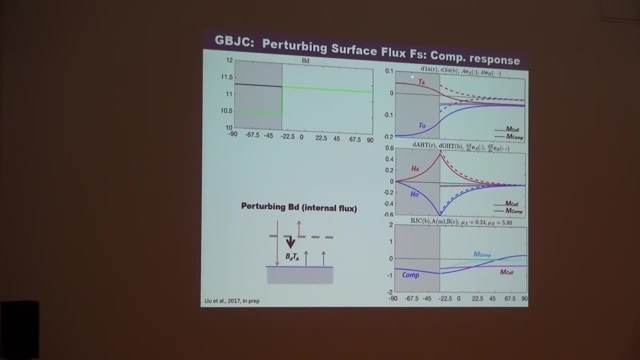 because ocean gain less heat, atmosphere loss less heat, so atmosphere warm, ocean cools And ocean-atmosphere heat transport opposite this compensation response, This ratio ocean divided by atmosphere heat transport is negative. But then this part: there's no perturbation. 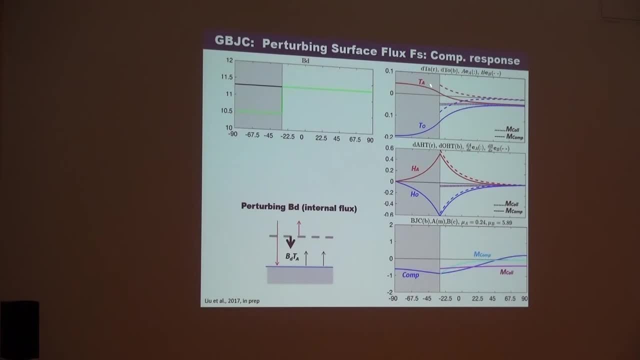 Everything comes from here. like I'm speaking here, whatever wave come out- high pitch or low pitch- coming from here. Here there's no forcing, okay, So you can. it's fuel propagation, So you can see this compensation response. 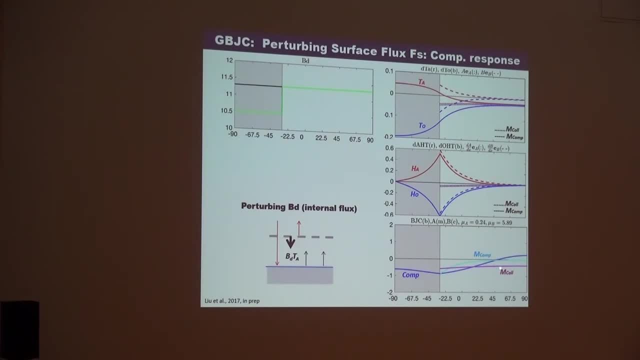 quickly damped, quickly damped, And actually here it become actually positive. So the ratio actually become positive. It become a collaboration response in the remote region, far from here. Now it's opposite, if I perturb it. 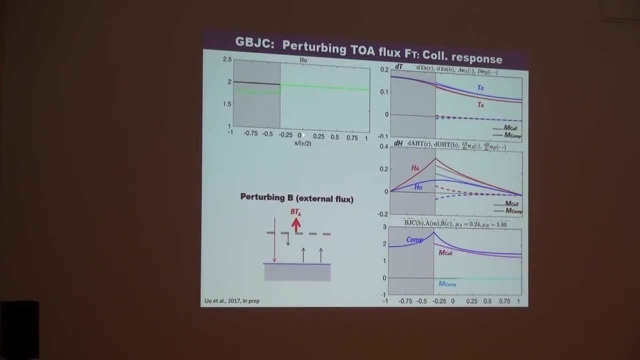 with top atmosphere heat flux. In this case I reduce a damping on the atmosphere on the top. So both atmosphere and ocean warmed up. Just I lost more. lost less heat on the top. everybody's happy, we just warm up. 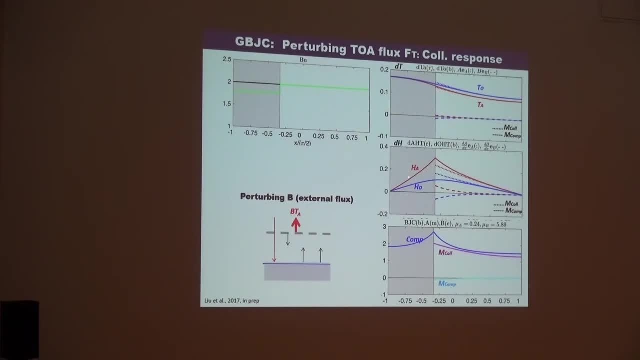 Once you warm up both atmosphere and ocean, produce heat transport towards the north. Now you look at this one heat. this response propagates far away. you know very robust all the way to towards this region And the Biettner's compensation is always positive, okay. 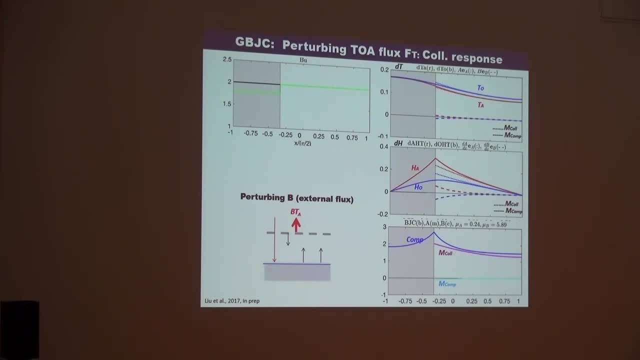 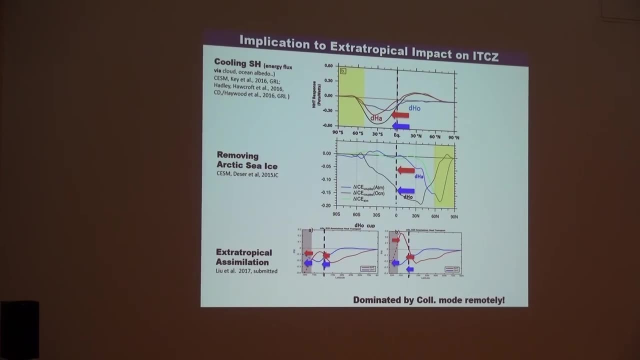 So it just shows that if you don't excite thermal heat line response, then the remote response is dominant by the, by the collaboration response. I think this explains, at least is a major reason- this couple GCM results. 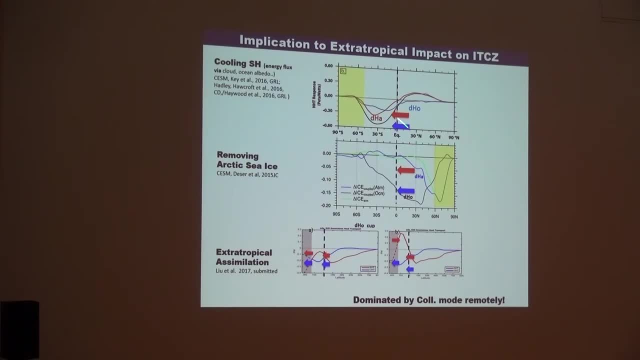 In this case you perturb south hemisphere and then end of the ocean goes the opposite direction. It's collaboration response. remotely Same thing for this: you perturb octant region. ocean and atmosphere go the same direction- the collaboration response. 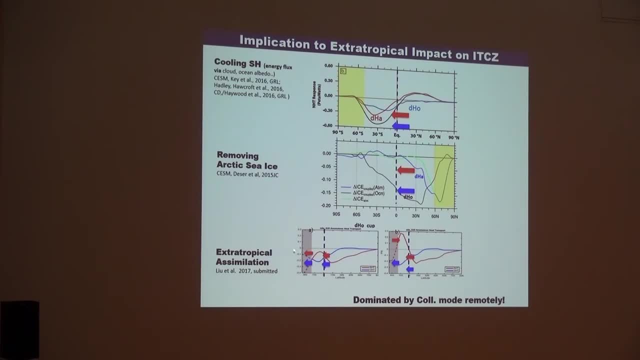 And we actually did another experiment in the fully couple GCM. it was for some other purpose, not for this purpose, but it happened. that will produce same direction of heat flux in the southern hemisphere. Then this direction you can see. 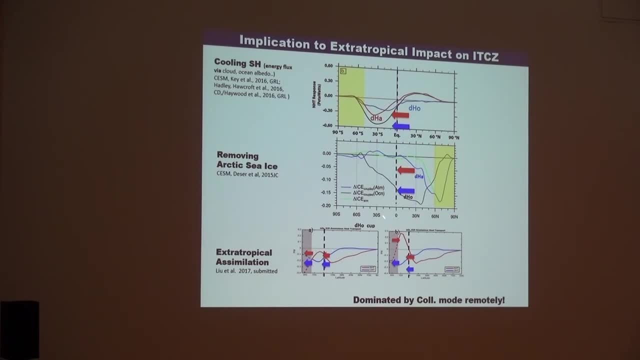 they all go the same direction. So this collaboration mode. In another case we produce opposite response of heat, flux, atmosphere, ocean in the southern high latitude, But then look at this region, Then they all go to the same direction. Initially the opposite direction. 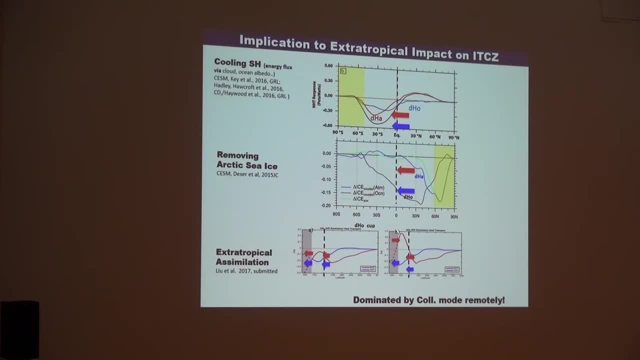 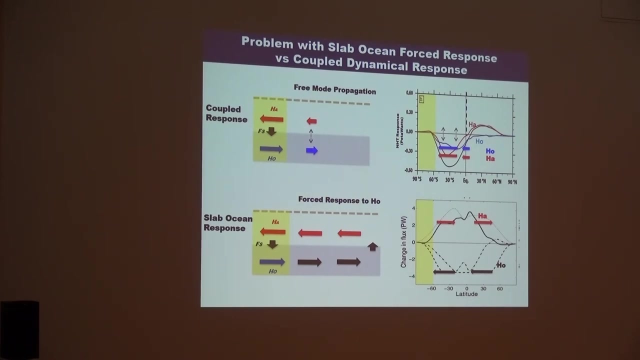 but later they damped out. the biogas compensation mode damped out, you're left with them going the same direction. So I think it's indirect proof in the GCMs we have Now in the slab ocean model it's very easy to change the ITCZ. 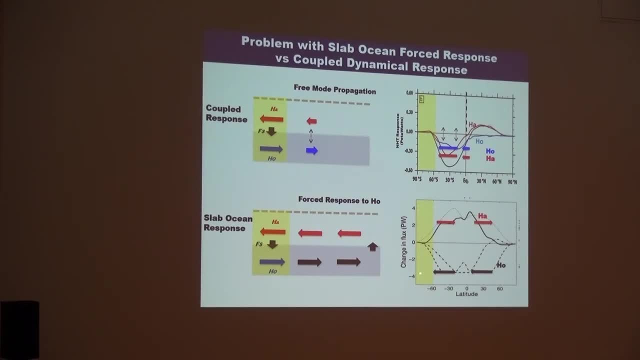 That was because in slab ocean model you prescribe the heat transport, So you sort of implicit assume I already have this remote propagation all the way through. Then it come from the surface. you perturb the atmosphere budget, then you change the ITCZ. 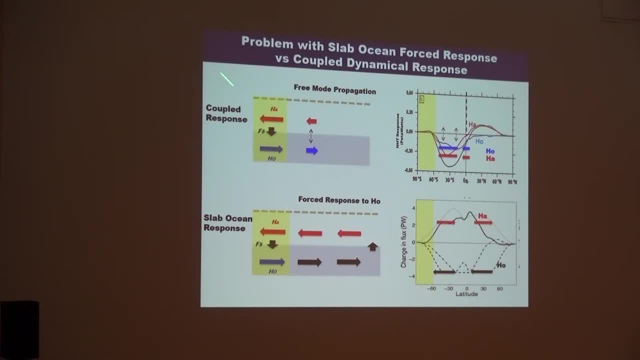 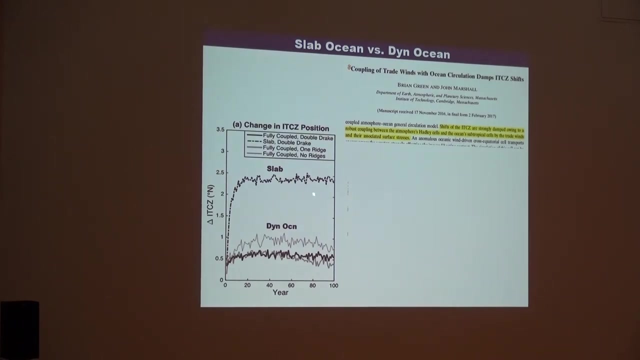 So that's in the slab ocean model, So in the fully coupled model. this actually perturbed high climate. It should become a fully coupled mode. Then the perturbation propagation becomes much more less efficient. And I think this is- I mean, this is a later paper after I wrote it- 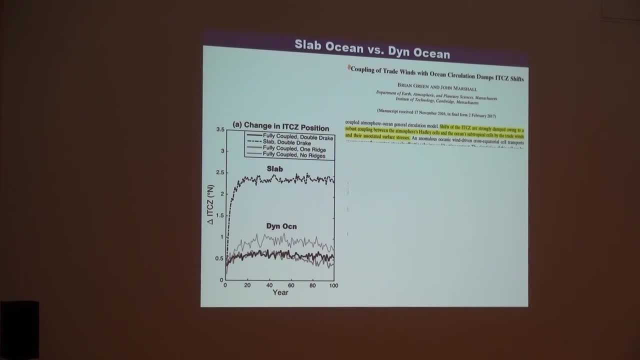 I submitted my journal John Marshall. they did experiment. They were doing fully coupled model. Then they perturb high latitude. They want to watch how much ITCZ changes. In slab ocean model the ITCZ moves 2 1⁄2 degrees. 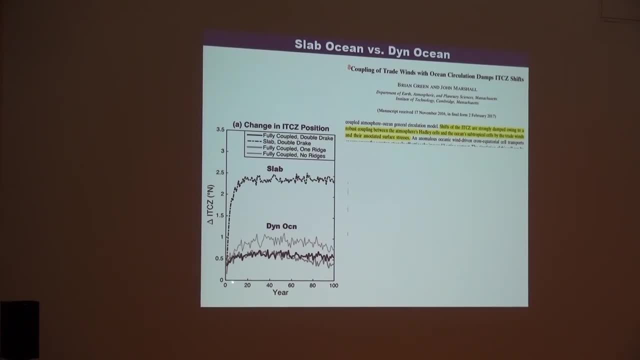 Exact the same change in coupled model: 1⁄2 degree, And they did specify there was a coupled ocean-atmosphere coupling. They were looking, diagnosing the coupled model. They found that there's ocean-atmosphere coupling there. 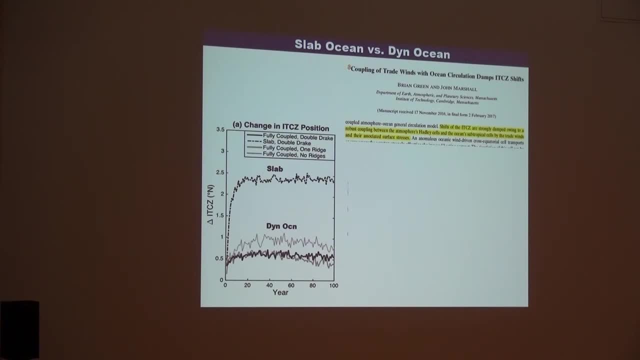 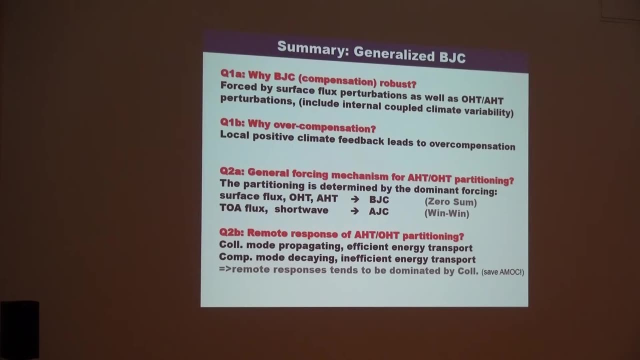 somehow trying to cancel this. So I think this can be explained with my simple theory in the first order. So here's a summary For generalized problem. it's compensation, which is really just. you perturb a climate system. how does the atmosphere, ocean, heat, transport respond? 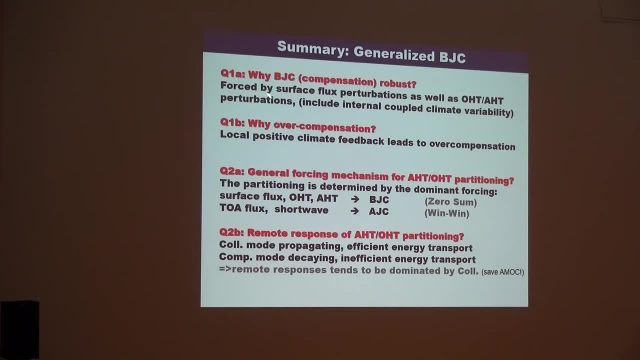 That's the general problem. okay, And so number one: if it's perturbed by ocean alone, then, as long as it's stable climate, it's always compensation, And in that case, if you have a local positive feedback, you can even produce positive feedback. 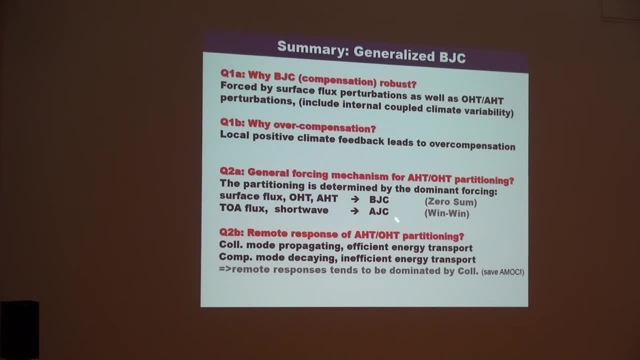 in global mean temperature change. But more generally it's that if you perturb a surface flux, dominant, If it's a surface flux, then you produce compensation response. Otherwise, if you perturb top-atmosphere response, then it tend to be the collaboration response. 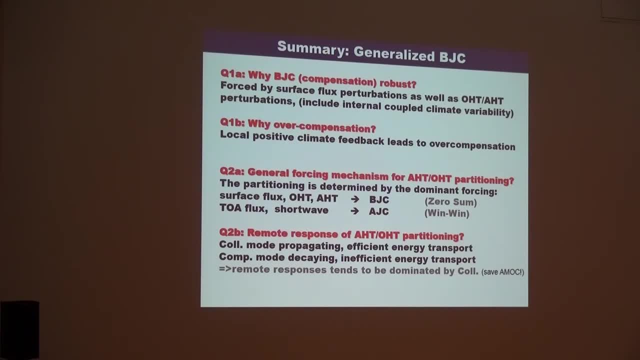 And finally for the remote response, the compensation mode is heavily damped by the interface air-sea exchange. It damped quickly So it's very hard for them to go away, But the compensation response is only damped by the top-atmosphere radiation. 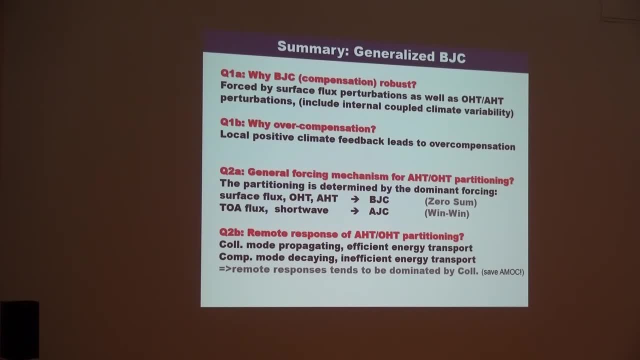 so they can propagate far away. So you start your production. you start your production, you start your cultivation, which is a mixture of compensation mode and the collaboration mode. But the compensation mode quickly damped. the collaboration mode propagates away far distance. 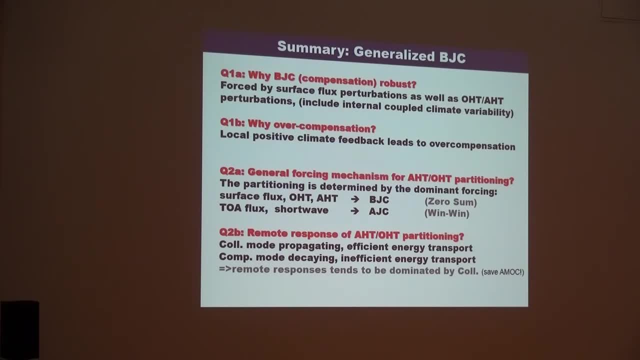 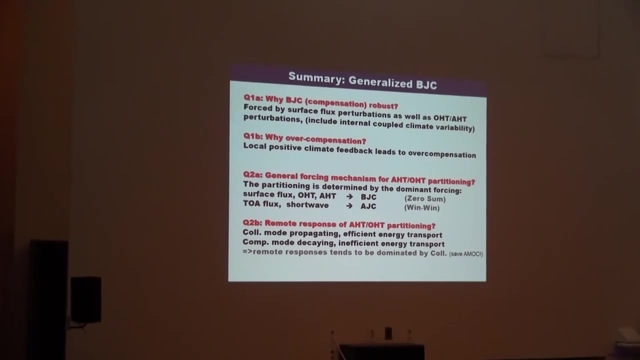 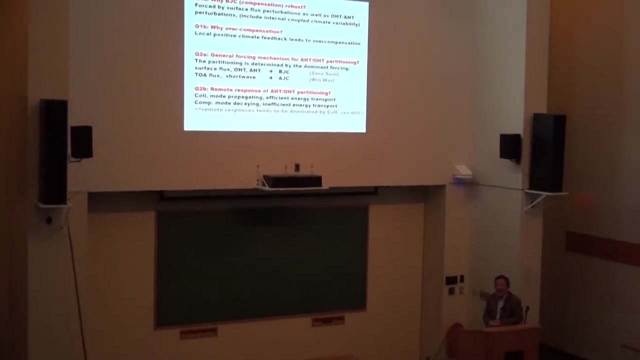 So in the remote region, what you observe actually is a collaboration response. That's my explanation of the GCM experiments. Okay, that's all. Thank you very much, Yeah, Yeah. So I'm surprised how much I enjoyed this talk when one of the punchlines is that some of my earlier stuff. 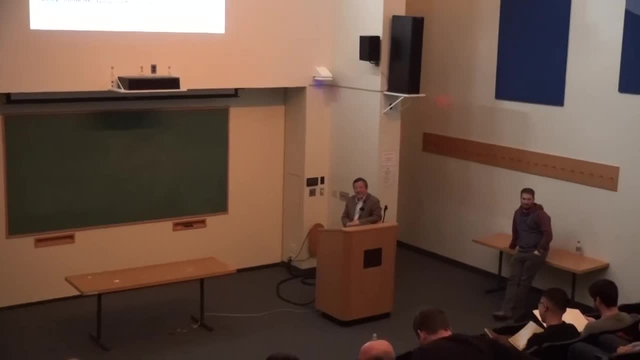 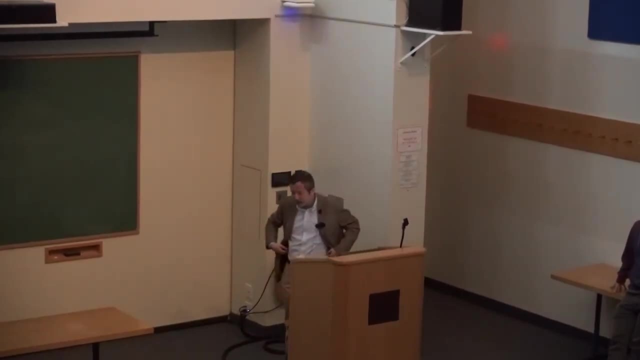 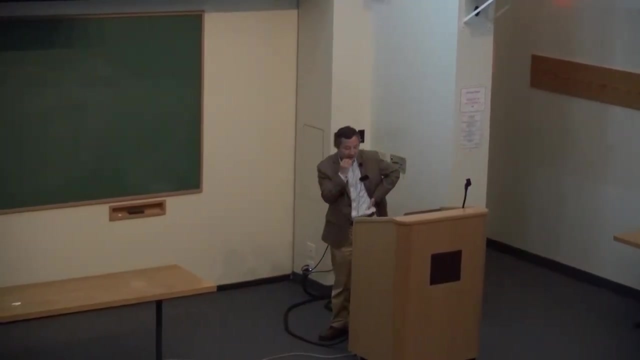 was quantitatively wrong. Well, not wrong, it's just stimulating. I just want to see if I'm delivering an understanding of the direction. So, in the experiments that Gen K did, where you showed the sea ice- both hemispheres- ocean clouds, sea ice- 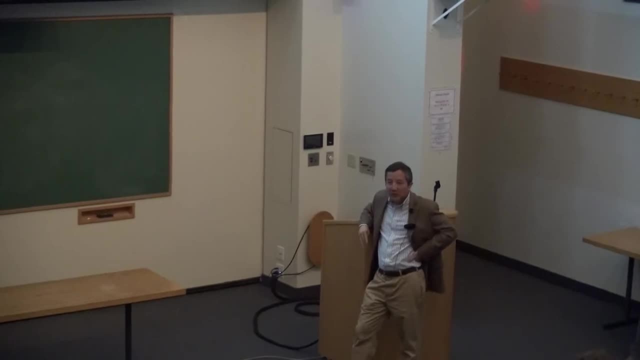 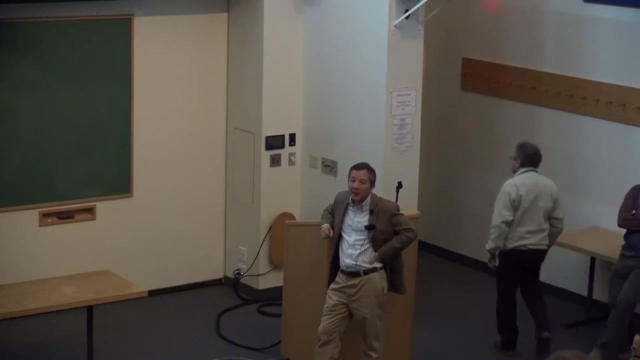 that's a coupled model. There's not much of an ITCZ response because the AMOC is not involved. Yeah, it's not too much perturbed, But in Zhang and Delworth, Ah yes, yes, exactly, Big ITCZ response because it does involve the AMOC. 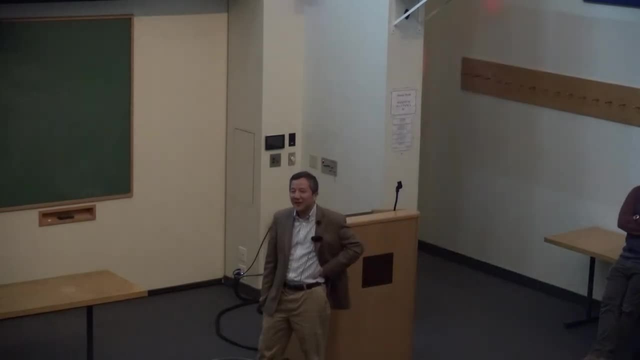 Yes, yes, yes, yes, yes, yeah. So in thinking about paleoclimes, we could still think about big ITCZ shifts happening, but they're more likely to happen only if the AMOC is observed. Yes, that's my conclusion. 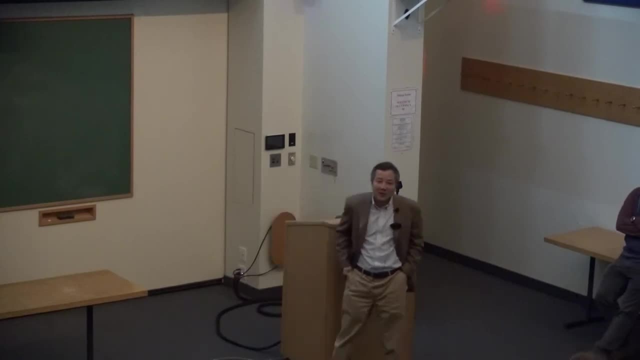 Okay, Yeah, yeah, That's cool. Yeah, yeah, Yeah, it was before I started this. it was just puzzling. On the one hand, I feel this is a fundamental problem, But I don't have a rule of thumb, you know. 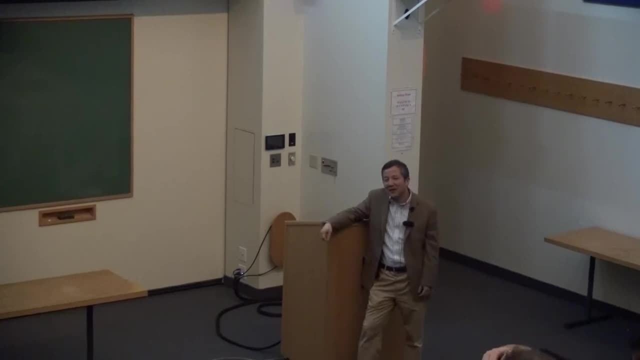 You see, some time happen, lots of time happen. And by the way, just another thought: Yeah, So in the slush kind of experiments there's almost always going to be overcompensation, Right? No, if you have local positive feedback. 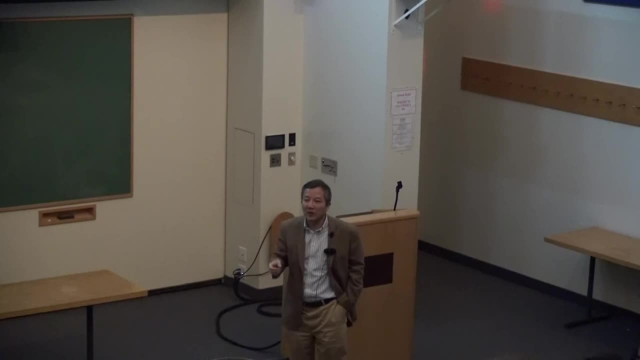 But there almost always is going to be local positive feedback- water vapor feedback and albedo feedback- And then that has to be well, in that region. you have to compensate the negative to become: yeah, yeah. If you have that, you could, you could. yeah, yeah, yeah. 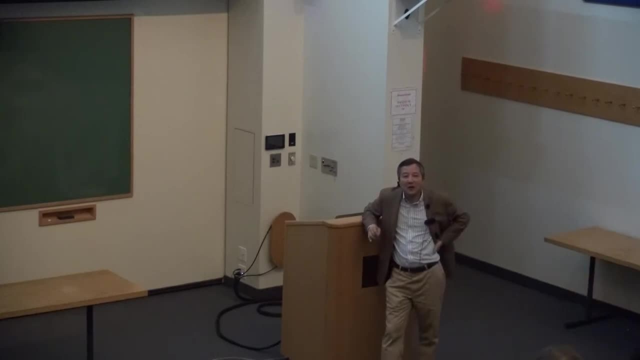 Yeah, Yeah, I didn't talk about that. You, basically I. we have a paper on the time variability part. Actually, let me just check on this. Well, the conclusion is that when the time scale is like about decadal- 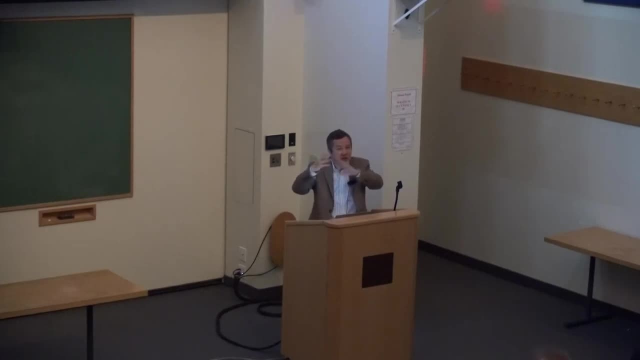 even longer time scale, then the solution is more. the compensation is more or less right. If it's inter-annual it doesn't work, Like any you know too, too fast it doesn't work. But it's long enough. when the transport start to the heat, storage is no longer. 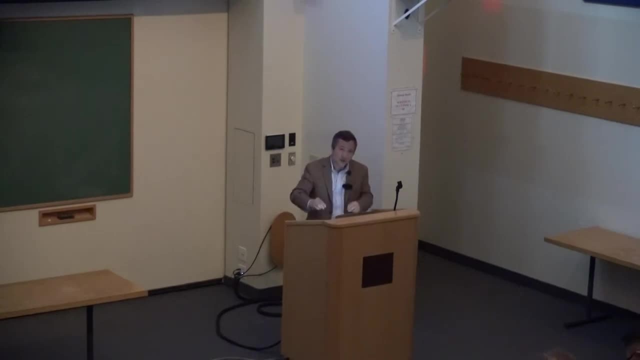 in a potion, no longer dominant factor, you will have them So. so this shows up in GCM experiments. I sort of didn't show that figure here. Okay, in GCM you can see that these are different experiments. 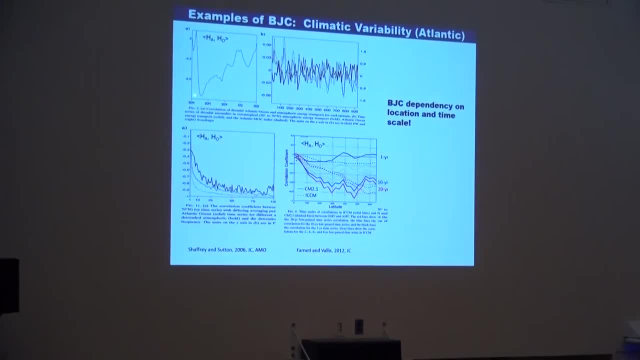 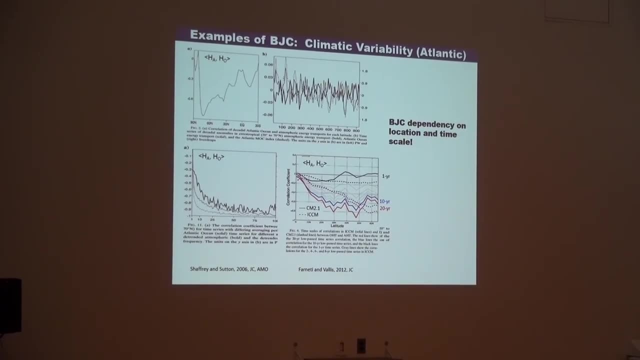 This is atmosphere-ocean correlation, heat transport correlation at different latitude. Okay, in this case you have them. this is a kind of variability In a just fully coupled ocean. you measure the ocean atmosphere, then you do a correlation right. this negative. 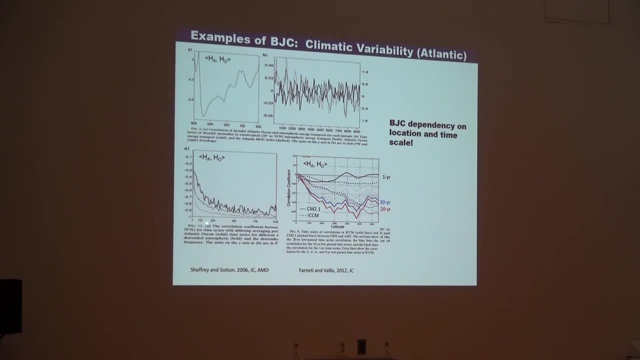 What I want to show is this: two: This is time scale, this time scale. So atmosphere-ocean correlation, This is time scale. This is time-ocean correlation at mid-latitude somewhere. You can see that if the time scale is very, very short, there's no compensation. 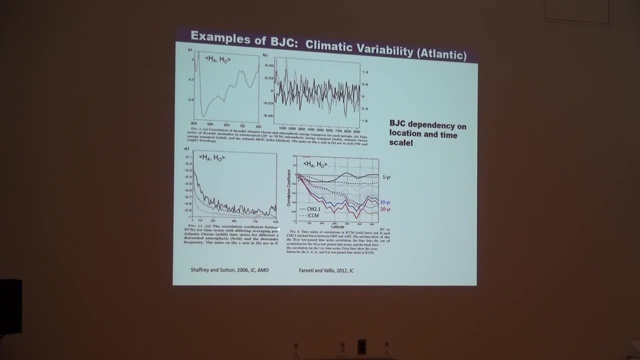 It's when the time scale become long, they become approaching the steady equilibrium response. So eventually you have the compensation response we talk about. So the solution will be it's equilibrium theory. So you have to have the system fully adjusted, not fully adjusted. 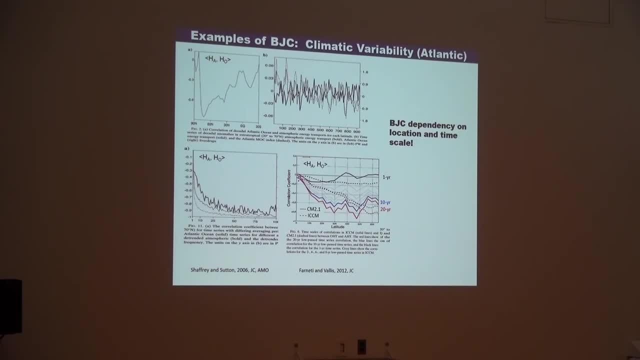 it dominantly adjusted, that then you could. you could work, And the qualitative The qualitative. it's also always true: Lower frequency the more likely the equilibrium solution is correct. But if you have very high frequency, this doesn't, doesn't even apply. 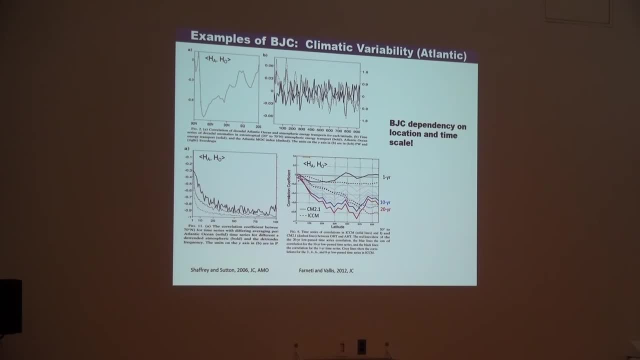 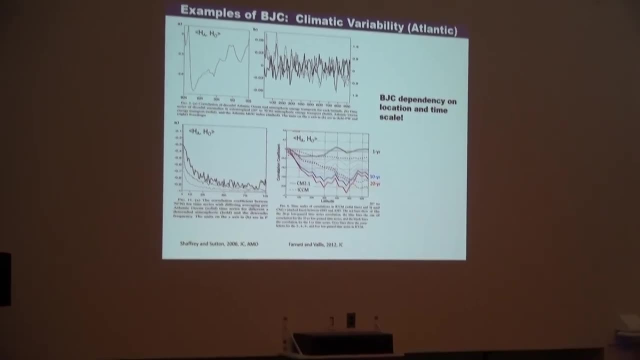 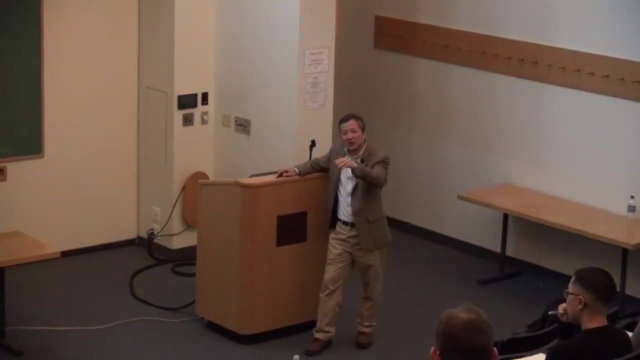 Yeah, And also for the paleo. you know, just the thing I always bothered, I always didn't quite understand before. you know, in the Cretaceous global warming, The ocean heat transport increase is one hypothesis Right. 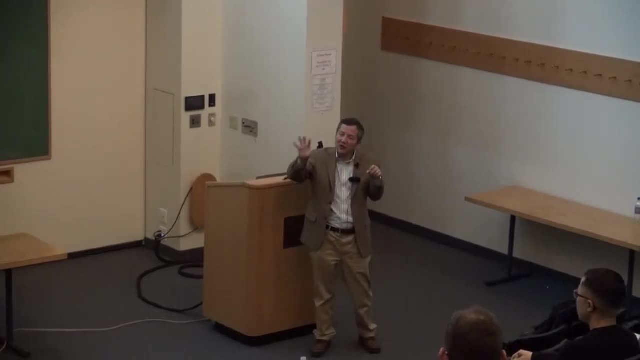 People say: But I always thought: well, you transport heat, you warm this here, But you cool this here. How can you get a global warming Now? here it's clear. Okay, If you transport heat to high latitude in the meantime, you have a positive feedback. 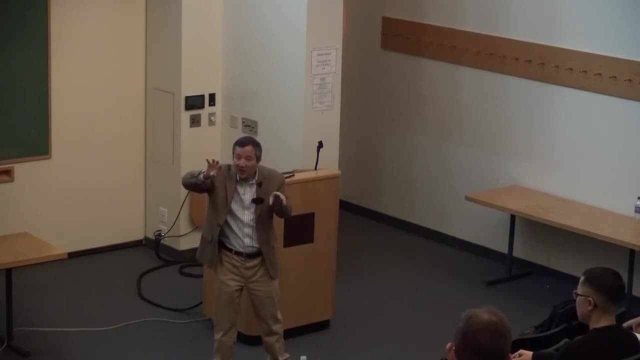 Like you know, some people that do a simple model. they want to have ectotropical positive feedback Because clouds change or whatever. Then, yes, You think about now the high latitude region. It's the region you generate extra heat. 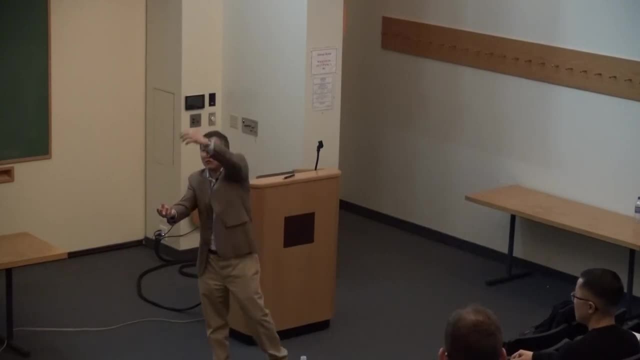 Because it's a positive feedback. So you give a little bit of heat, then you produce more heat. you come back, you warm everywhere, Then you go together. Okay, It could be the opposite Because, uh repeat, Hamburg used the same thing, but focusing on the tropics. 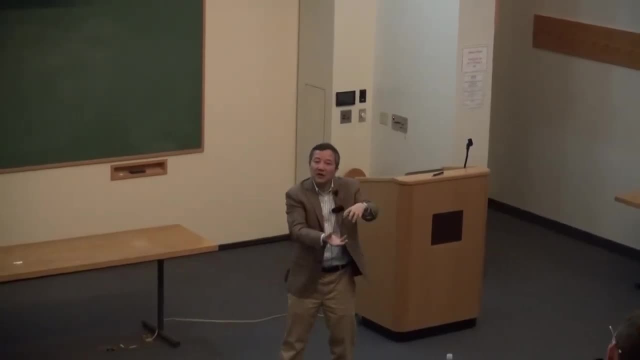 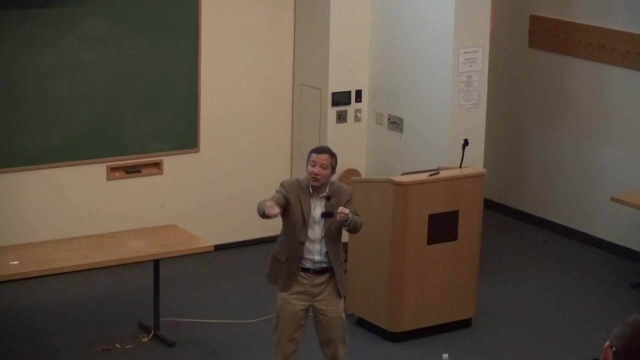 It could become the called a thermostat Tropics positive feedback. but you transport heat away. you lose heat. You lose heat. so you, you radiate heat from subtropics Where you have a stronger damping. So instead of damping the tropics, you're damping the subtropics where there's a stronger damping. 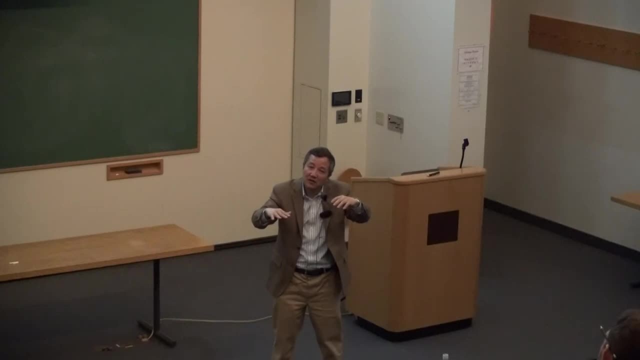 So then, the global average. that's why you can stabilize this. Stabilize Even though positive tropics, you can have positive feedback. So you still don't have a runaway greenhouse gas because global mean is still stable and you can still damp it here. 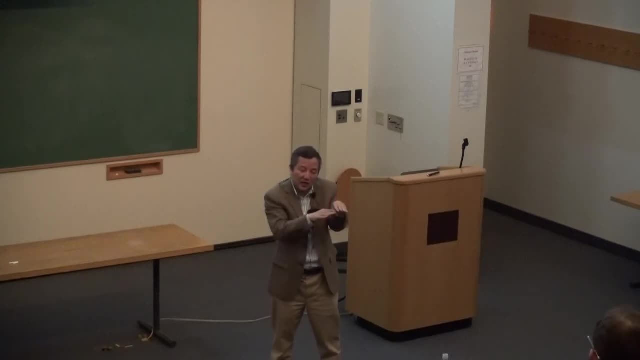 In this case, because you transport heat this way, then you lose some heat in the tropics, But it's positive feedback, So you lose a little bit of heat, you lose more heat. Okay, So then you can stabilize the global mean. 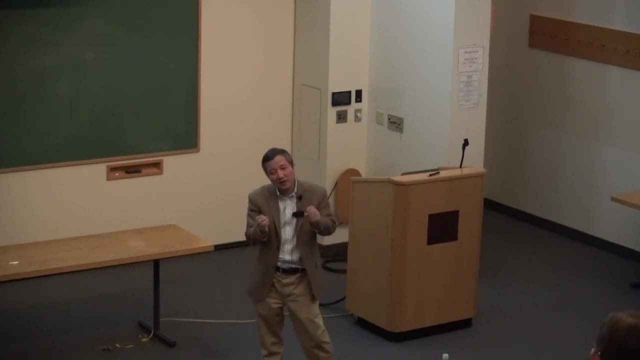 Not just tropics Stabilize the global mean. So it really depends on heat, transport and local feedback, the relative position. I think I don't think people have thought about this so carefully and this just make it more. this point, relation to global mean- just make it more explicit on this part. 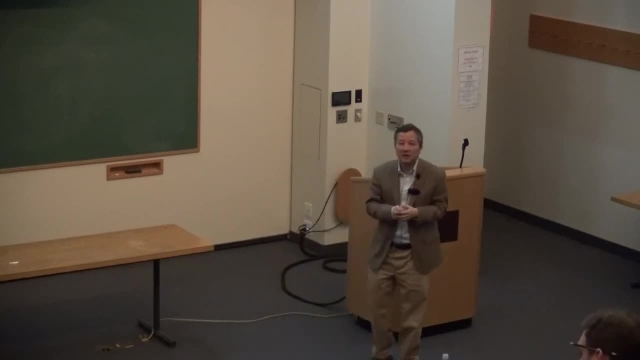 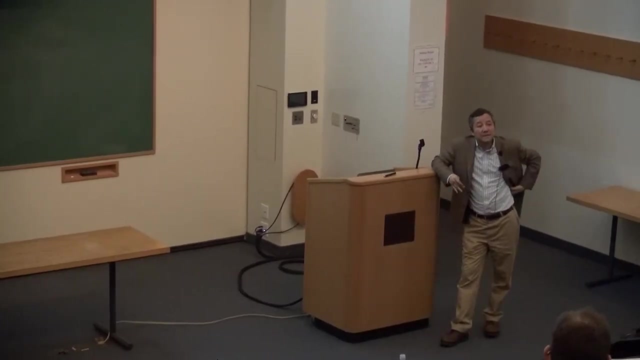 Yeah, Okay, Okay, Thank you. Yeah, You know, you can kind of take a look at, uh, how tasks and I, Okay, That's true. Uh, yeah, So now, Okay, I'm not sure if that conclusion is right. 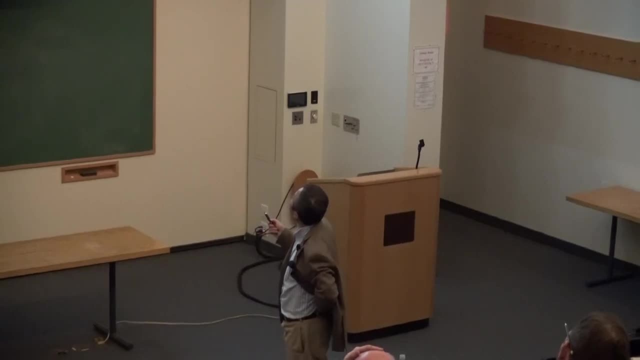 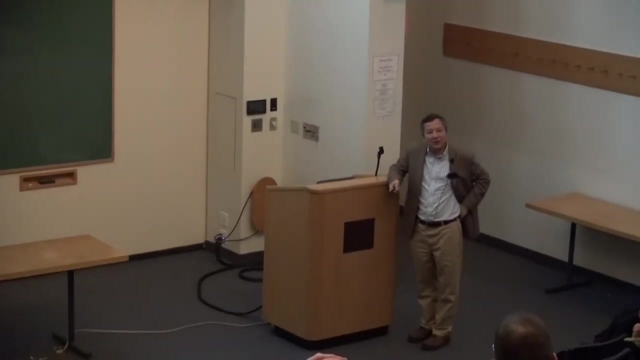 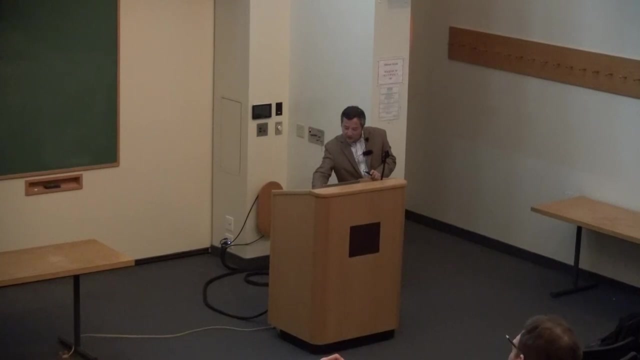 Let's look at this. OK, so this time scale, Yeah, I don't know if that conclusion is right. High latitude is higher. I don't know if this is right. It's not very obvious to me because I didn't divide this here.